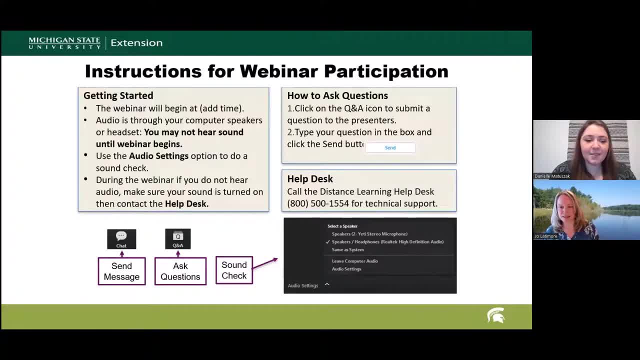 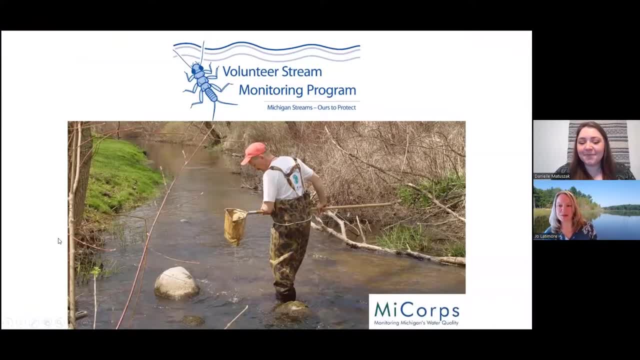 Miroupell, 1. Alright, so the Michigan Clean Water Core is Michigan's volunteer lake and stream monitoring program And we have three key programs that make up this initiative across Michigan. One is our volunteer stream monitoring program that engages volunteers across the state in collecting invertebrates- insects from streams. 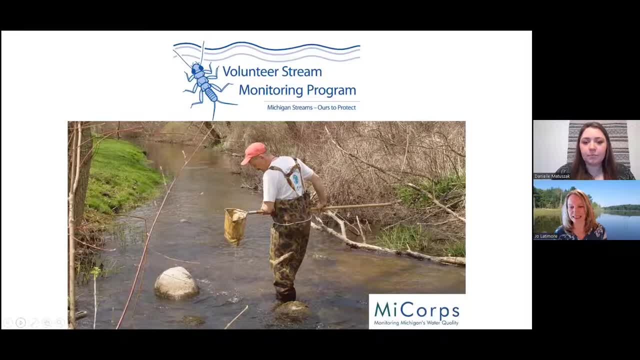 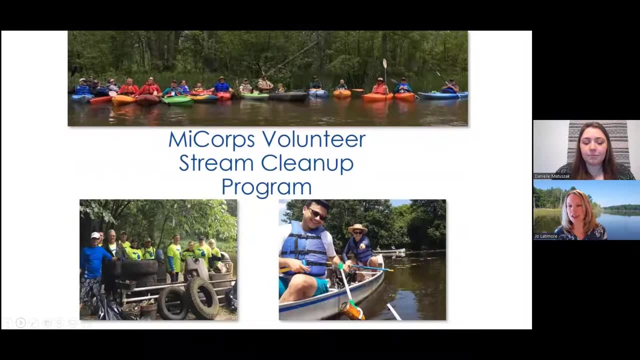 to better understand their health and assess their habitat quality. Next slide: We also have a volunteer stream cleanup program that we support, where local governments can apply for funding to host stream cleanup events to remove trash and garbage from the streams and rivers in their communities, And currently we are accepting grant applications for both our 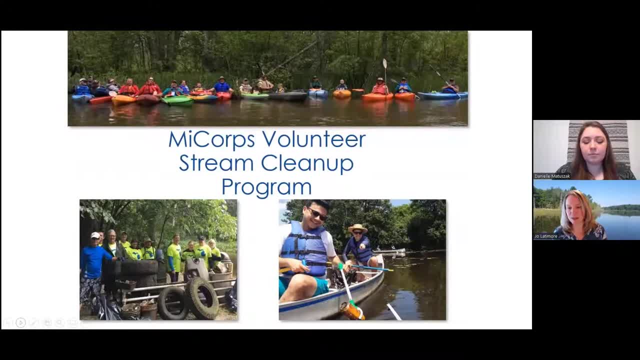 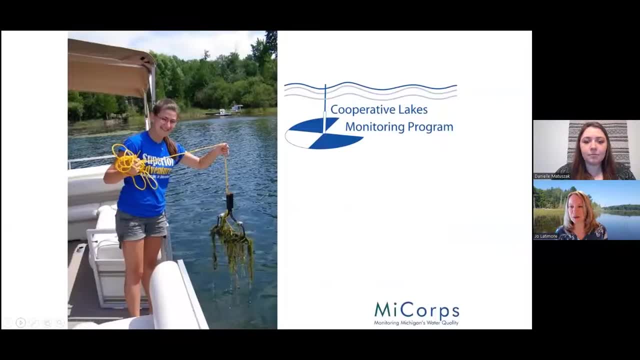 stream monitoring program and our stream cleanup program. You can visit our website for more information on that. Next slide And the third and final component of myCORE is the Cooperative Lakes Monitoring Program. This is our statewide lake monitoring program where folks around the state monitor more than 300 lakes across Michigan every year for water quality. invasive species. 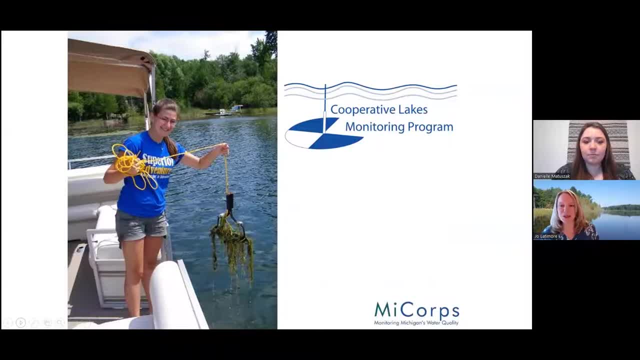 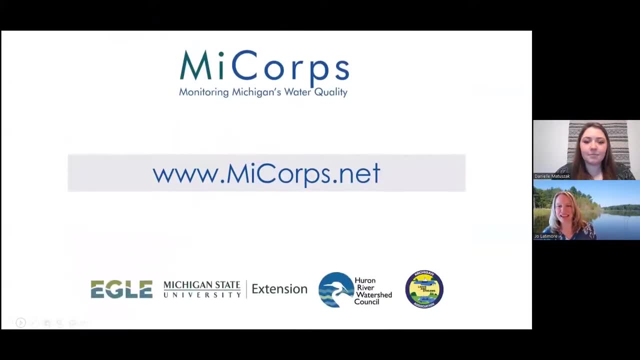 and much more So. regardless of whether your interest is streams or lakes, we have a program for you. Next slide, please. You can learn more about the myCORE program at myCOREnet. myCORE is a program of the Michigan Department of Environment, Great Lakes and Energy. MSU Extension: the Huron River Watershed Council. 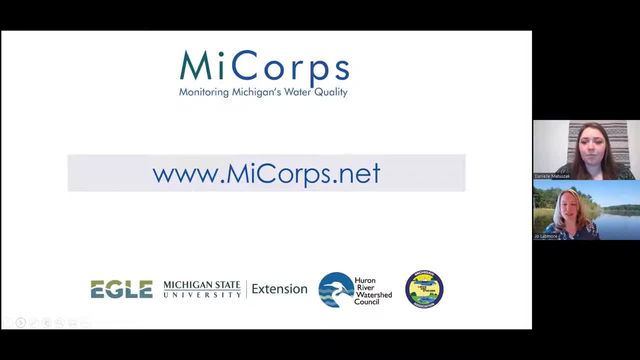 and Michigan Lakes and Streams Association. Now, with no further ado, I'm excited to introduce our main event, the reason that you're all here. I'd like to introduce Danielle Matuszak. She is a master's student in the Department of Fisheries and Wildlife at Michigan State University. She works in 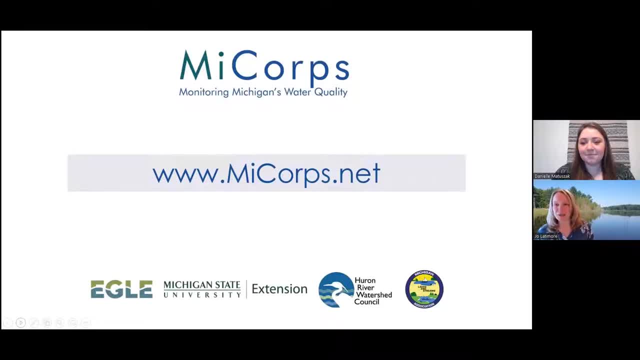 the Data Intensive Landscape Liminology Lab, where her major advisor is Dr Kendra Sharavelo, And if any of you were able to join us for the last Michigan Inland Lakes Partnership Conference back in 2020,, Dr Sharavelo was one of our keynote speakers. I know a lot of you enjoyed. 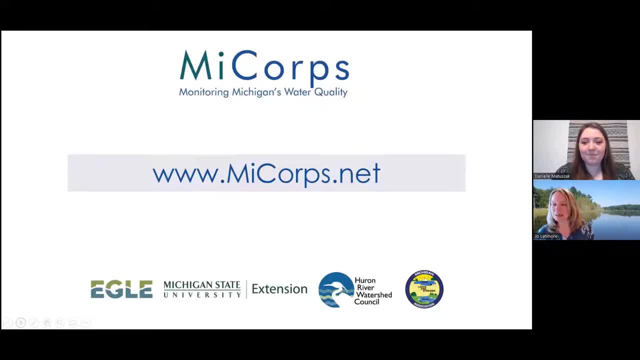 seeing her. I know Danielle is going to tell us a little bit about herself and her background, So I'm going to hand the screen and the microphone over to you. Danielle Matuszak datasets. representatives for the Michigan Mchwartar Lakes and Lake. Mountains National Science Foundation. Okay, see you. Susan will breakdown first, then Sharavelo will talk about the resources for opportunities for the organization. Again, she was involved in this program and she shares her leadership experience as a product. Thank you, guys. You have definitely a lot to Himayat and care for rankings and data intensive landscape limnology. 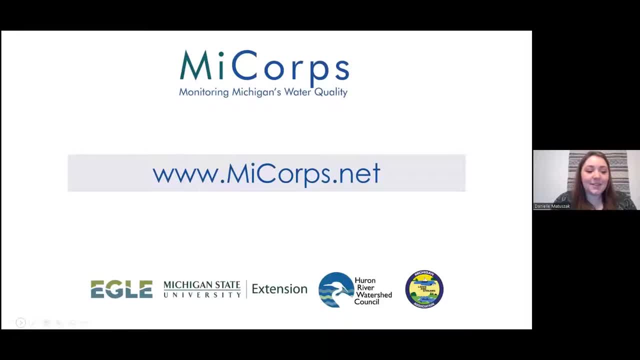 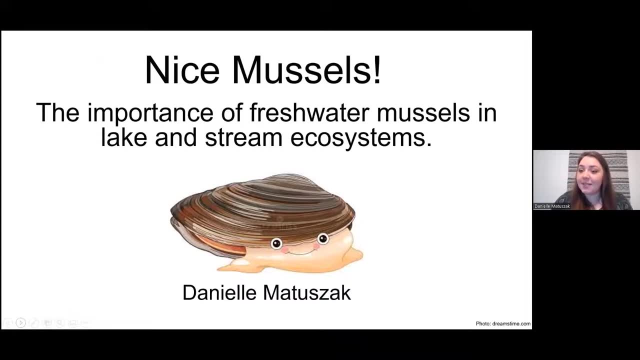 such a nice introduction, So yeah, so, as Joe mentioned, I'll be presenting on freshwater mussels. As you guys saw when you registered, the title of this presentation is Nice Mussels: the importance of freshwater mussels in lake and stream ecosystems. And so, to give a brief, 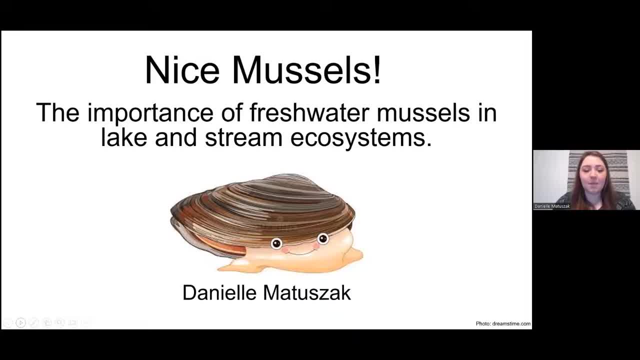 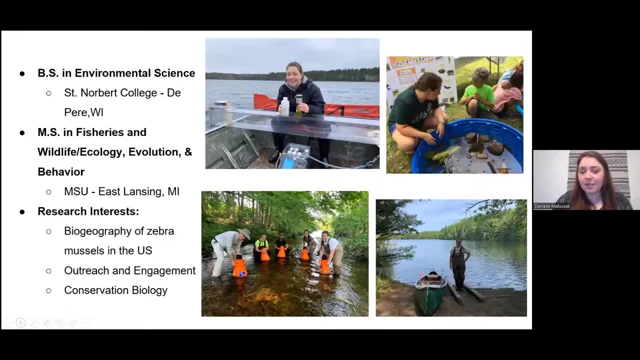 overview of kind of who I am, my research and my passions for science. So I got my bachelor's degree in science at St Norbert College in De Pere, Wisconsin, in environmental science, where I had the fortune, to the good fortune, to be able to work for several different research labs. 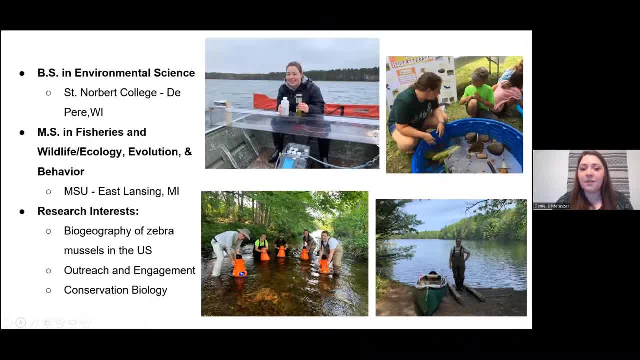 as well as spend a summer working for UW Madison's Trout Lake Field Station in northern Wisconsin, where three of these photos are from. While I was a undergrad, I was able to work with outreach doing. the pool photo there in the upper right shows me. 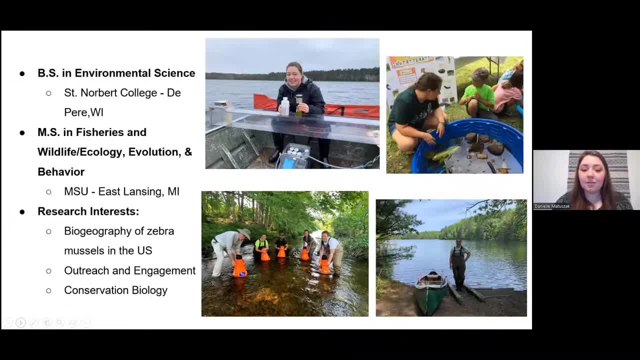 you can see the pool photo there in the upper right. shows me. the pool photo there in the upper right shows me interacting with the public for Trout Lake Station doing outreach, educating the public about different invertebrates that are found in the lakes and streams surrounding this. 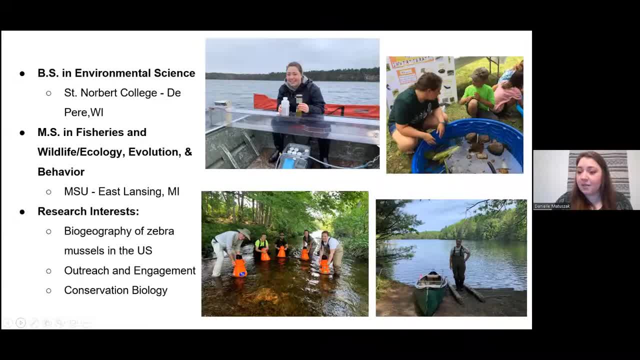 station. I also have helped with freshwater mussel surveys here in Michigan And I've also done individual projects while I was up at Trout Lake and did a undergraduate senior thesis on the impacts of PCB dredging in the Fox River in Green Bay, Wisconsin, on Mac. 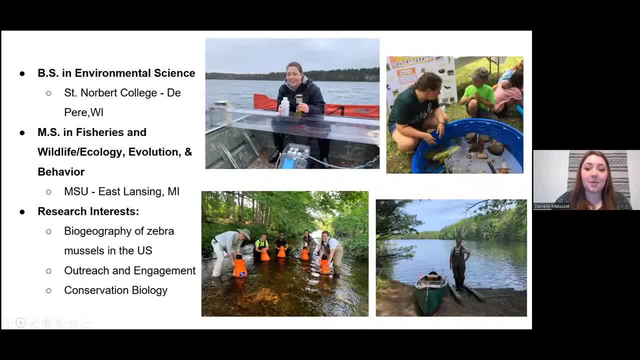 Greenberg populations. And so, as Joe mentioned, I am currently a masters student. I anticipate defending my research and my thesis this coming May, which is exciting with that deadline coming up, And so I am getting a dual degree in Fisheries and Wildlife, as well as Ecology. 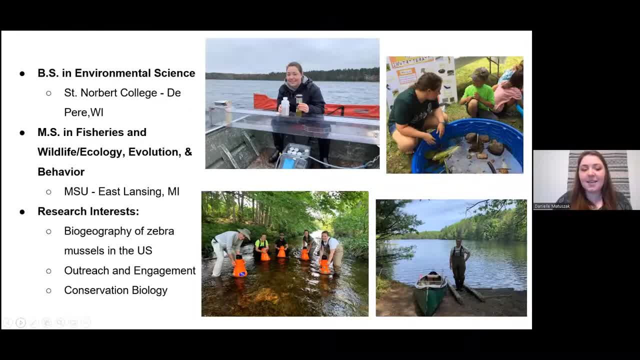 Evolution and Behavior right here at MSU in East Lansing, And to go a little about my research interests. my specific thesis research involves the biogeography of zebra mussels in the United States, and so zebra mussels are invasive species and I'll touch on that a little bit towards the end of 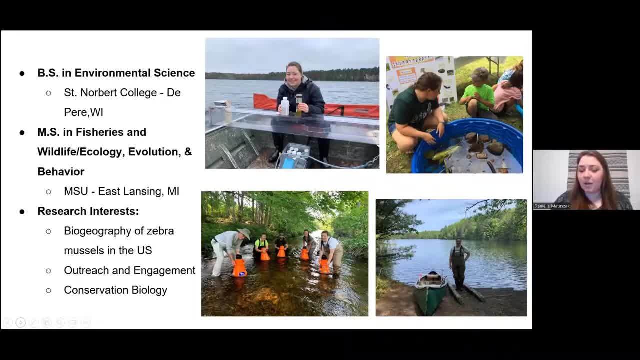 this presentation and then also, I'm very passionate about outreach and engagement, as is evidenced by being one of the key people putting on this webinar series and doing research. outreach and engagement from research and such in the past, and then broadly conservation- biology- is a passion of mine. I believe that we need to conserve and protect our natural waterways and landscapes. 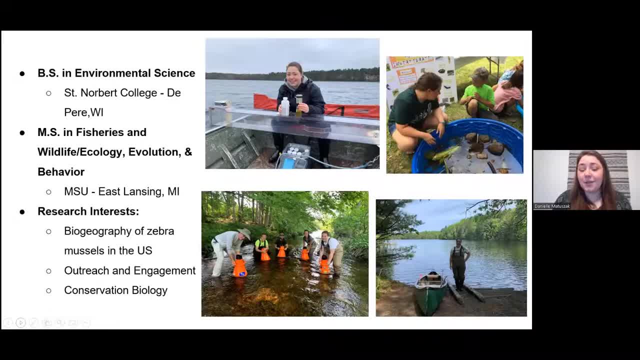 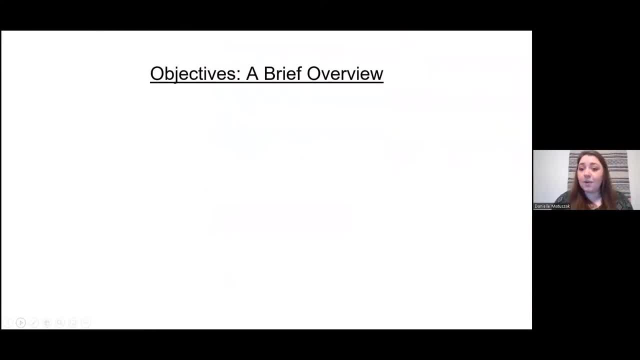 for future generations and for the organisms that call them home. and so, to start off, I'm just going to give a brief overview of kind of three main topics that I'm going to be discussing today in this presentation. the first is the general biology of freshwater mussels. I'll give an introduction to 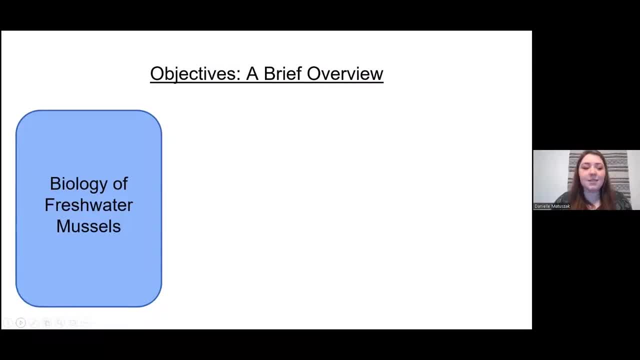 their life cycle, where you can find them with their habitat, those kinds of things, and then I'm going to follow up with the threats to those native freshwater mussels and then I'm going to talk a little bit more about how we're going to. unfortunately, native mussels are quite threatened in North America and in Michigan. 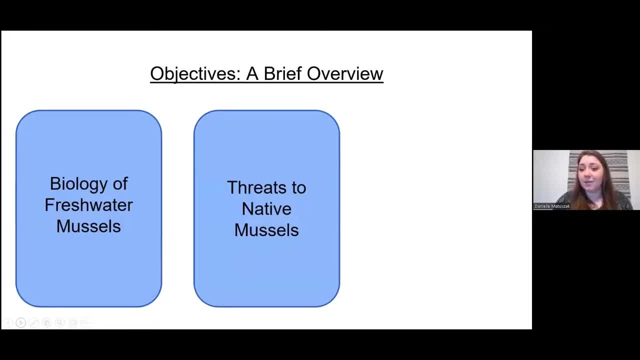 and so I'll go over a couple of the things that are threatening those native mussel populations. and finally, I'm going to talk a little bit about the conservation of freshwater mussels and what the United States and Michigan is doing to conserve and protect our existing freshwater. 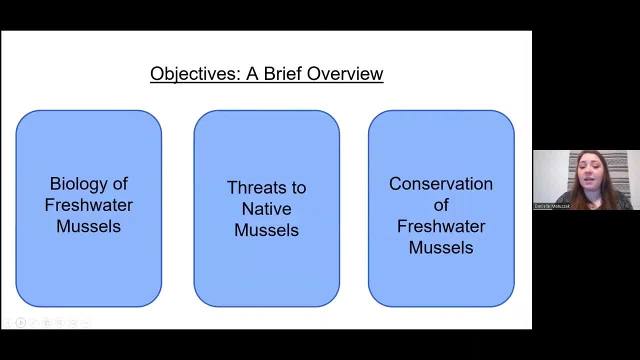 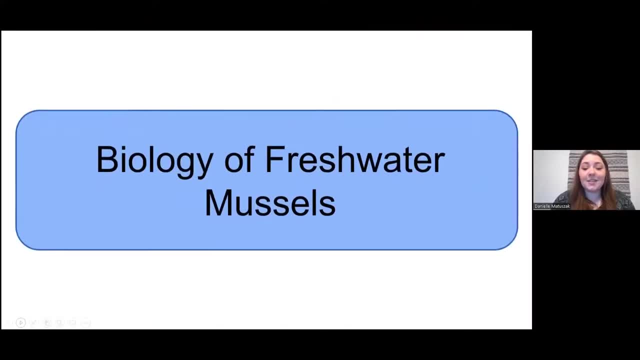 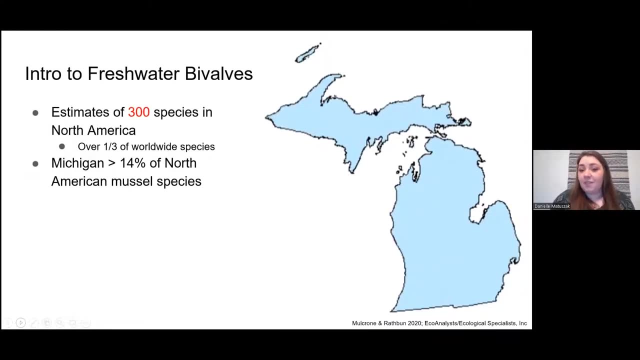 mussels, as well as potentially introducing freshwater mussels back into areas where they previously weren't. so, to start off, as I mentioned, I'll start with the biology of freshwater mussels. freshwater bivalves, freshwater mussels are very common throughout the world and in north America. 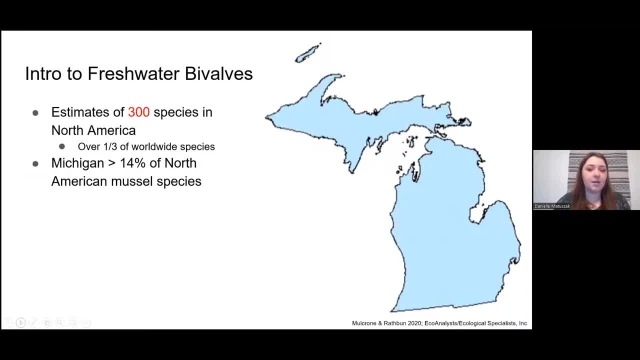 there is an estimate of about 300 species in North America alone, which makes up over a third of the species worldwide. so north America has quite a high diversity of freshwater mussels and Michigan alone has four over five million freshwater mussels, 14% of those American mussel species. So you're able to find upwards of 43 different mussel. 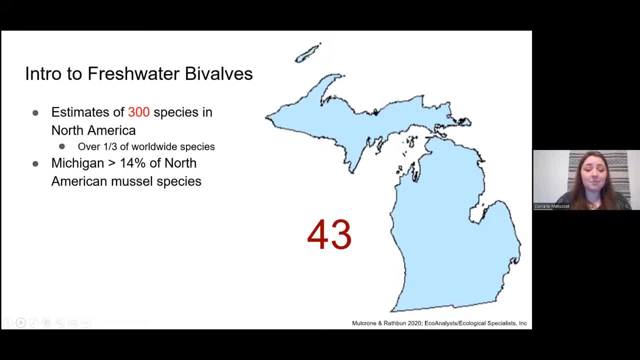 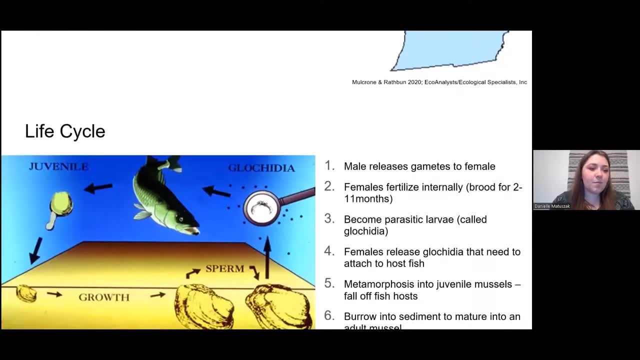 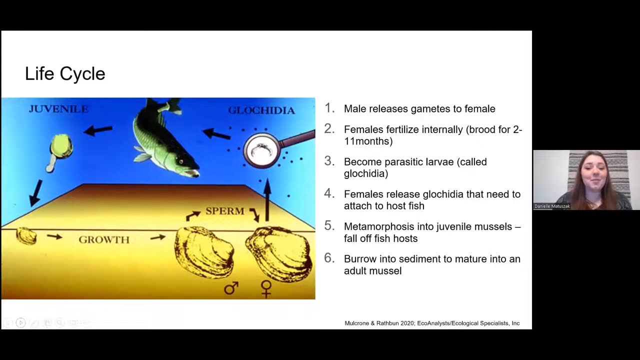 species throughout the Upper Palinsta and Lower Michigan, which is incredible since it has such a wide diversity for just one state. And one thing that is quite interesting and I find fascinating about freshwater mussels is their life cycle. Many people may not know this, but freshwater 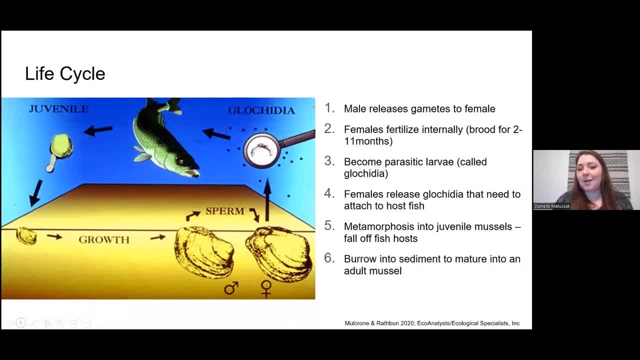 mussels actually have a parasitic phase, And so I'll quick walk through their life cycle, but that parasitic phase is key to their survival. So the way this goes, it starts out with male and female mussels. The male will release gametes into the water, into the female, where the female 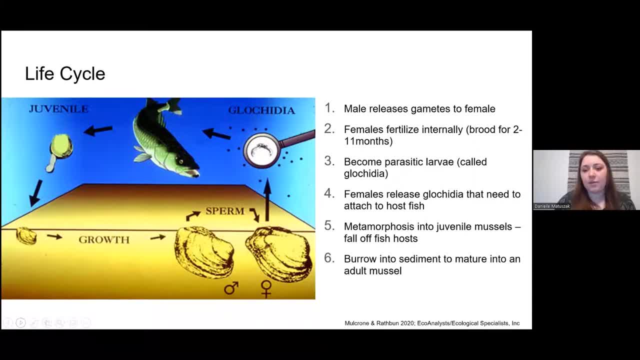 will fertilize internally and brood for about two to 11 months. Once that brooding period is over, those larvae are becoming a parasitic larvae called gochidia. When they have reached that parasitic phase, the females will release those larvae into the water. 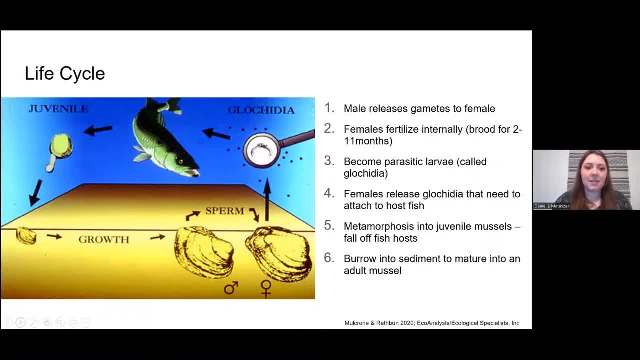 where they need to attach to host fish. This is that key parasitic phase. Many species of freshwater mussels require specific species of host fish for them to attach to and live in the gills of in order to reach their juvenile stage. Once a parasitic larvae, the gochidia have attached. 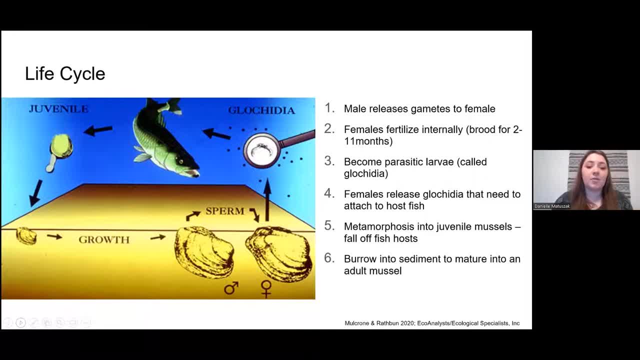 to a host fish. metamorphosis occurs where they go from a parasitic to a host fish. When they reach a certain size and a certain stage in that juvenile they will fall off the fish's host gills which will run along the sides there and they will drop into the bottom of a 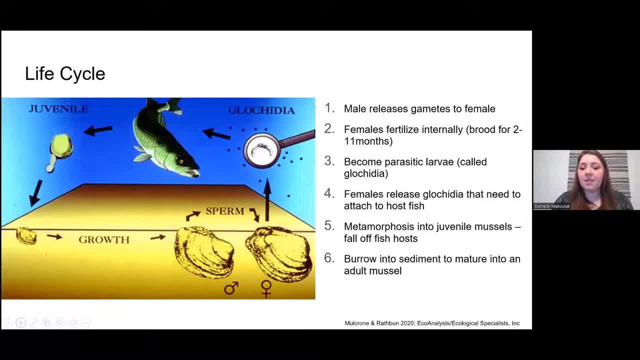 stream or lake, where they'll nestle down and burrow into the sediment to then mature into an adult mussel. Then, when those adult mussels are mature, the life cycle starts over again, starting with the male releasing the gametes to the female, and so on and so forth And so. 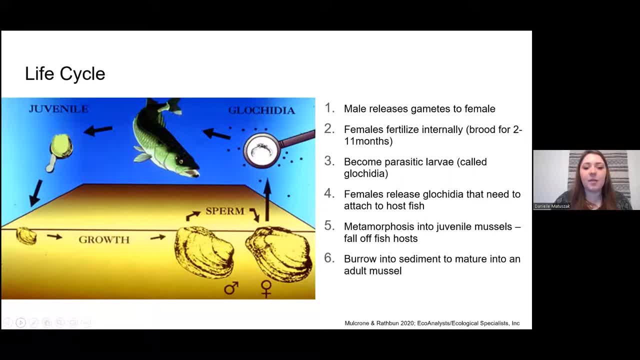 when I first was starting to look into research and become familiar with freshwater mussels, I simply assumed that they were just a mussel. They released their gametes into the water, fertilized that way, they dropped to the bottom and go. But that's not the case. They actually. 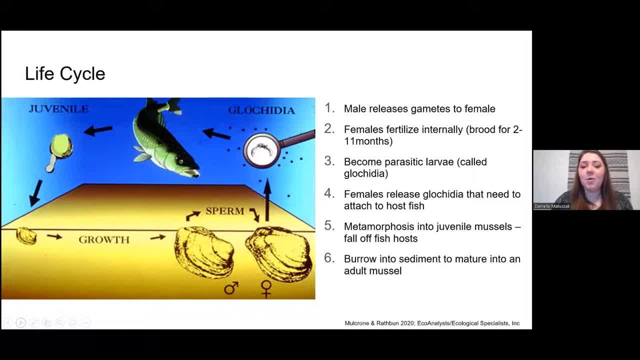 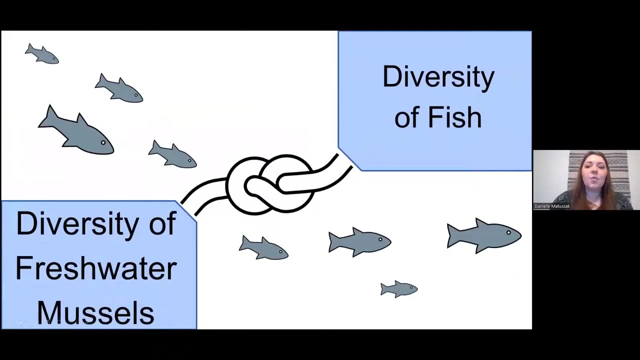 have a very complex and interesting life cycle with that parasitic phase- And I'll touch on that through a good part of this presentation about the importance of those host fish and that parasitic stage- And so one key thing that I want to emphasize is that the diversity of the freshwater mussels, that 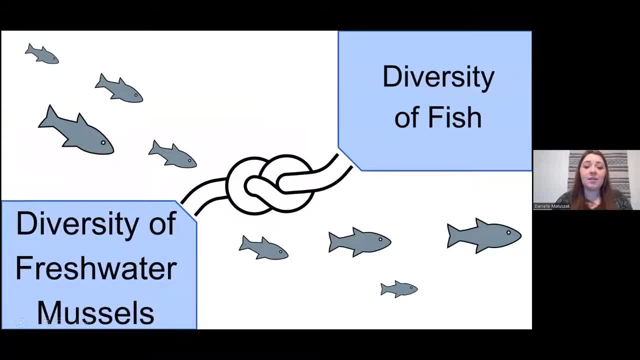 we have in lakes and streams throughout Michigan, throughout North America and throughout the world are very much dependent on the diversity of fish in those same ecosystems And that if a species of mussels does not have its specific host fish in its ecosystem, that can cause their reproduction. 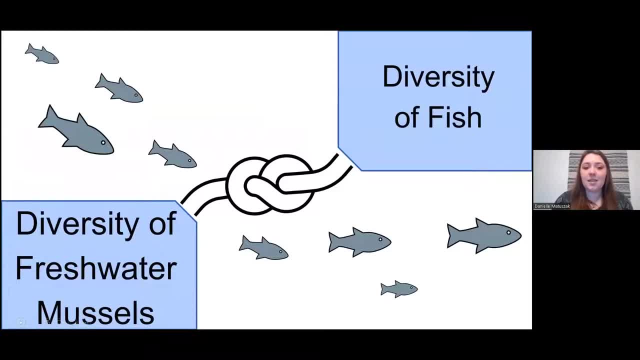 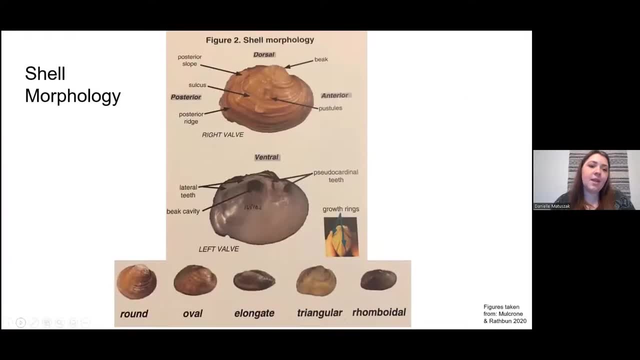 and the sustaining of that population to decrease. So you can see that the number of species, one species in a species of species- may be very, very small and it can become quite complicated and may lead to the decline of that population. I'm going to quick go over a little bit about shell morphology. I won't touch on it. 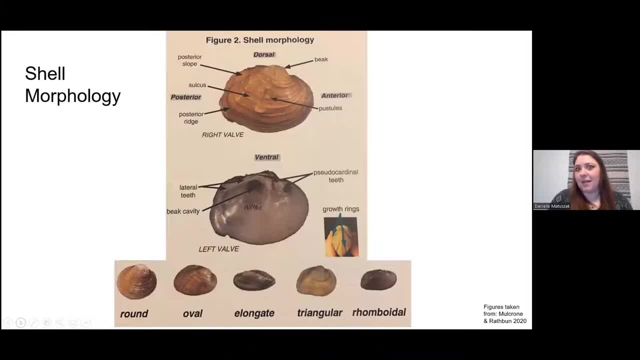 too long, since it can get quite complex. but when it comes to freshwater mussels, there are five kind of main shapes that you can find them in, And you may have seen some of these in your sampling that you have done in the past or may see them in the future. So we have the round ones. 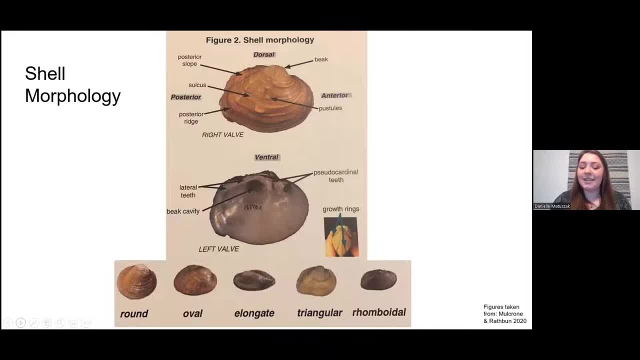 we have the oval, elongate, which are quite longer and skinny, and then the triangular ones and then rhomboidal, and so these five different shapes kind of make up the general population of freshwater mussels. most freshwater mussels fall into one of those shape categories and the shape and size are. 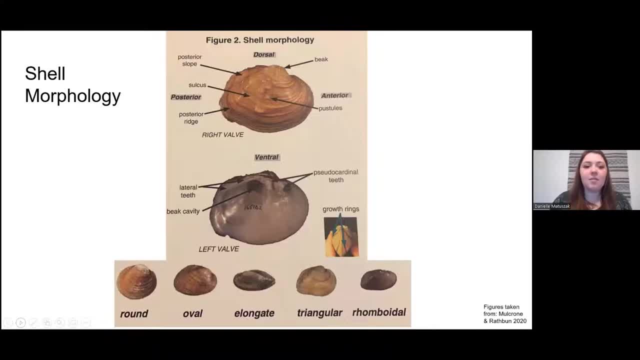 key things when it comes to identifying freshwater mussels. a couple other things: the morphology: you can see the above diagram. there shows a couple different identifications. so you have the beak of the muscle, you have the beak cavity, lateral teeth, ridges, all of these things, and so i won't. 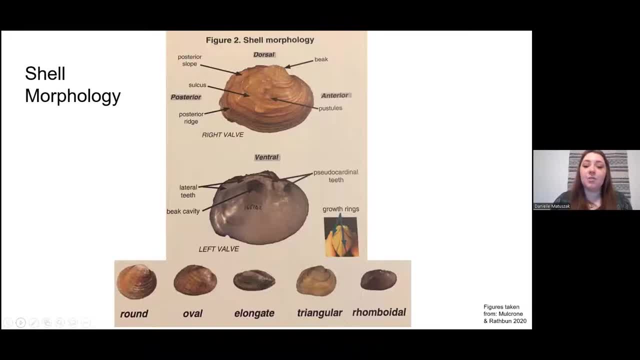 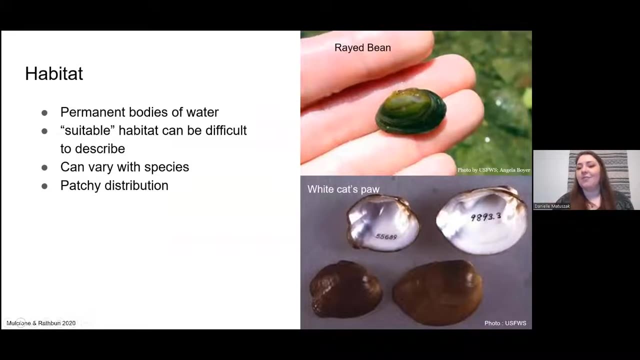 get too in depth, but these are some of the key areas that you use to identify freshwater mussels- not only their shape, but a lot of their general shell morphology as well, and so, as i said, i'm going to give an overview of their biology, and that includes their habitat. 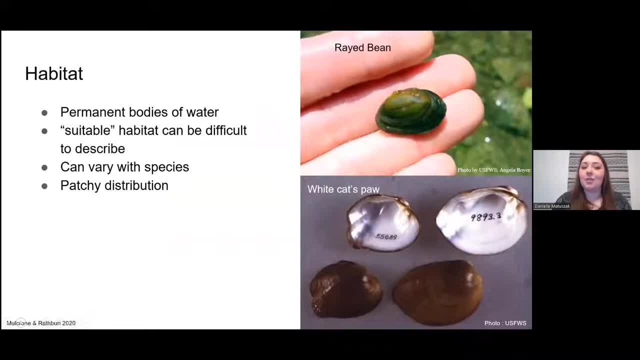 where do they like to make themselves at home, and so in general, they like permanent bodies of the water. so if you have a body of water that evaporates during the summer but then comes back in the spring or in the fall, you won't find muscles there, since they do need to stay submerged. 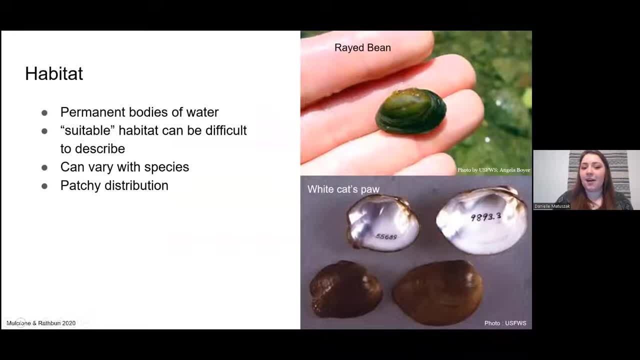 however, finding suitable habitat or identifying what a suitable habitat is can be quite difficult to describe, as it can vary greatly between species and between regions within the united states, north america and worldwide. i have pictured here on the top, a raid bean, uh freshwater muscle, quite similar to a freshwater mussel, and on the bottom, there, we have a white cat's paw as well, which has 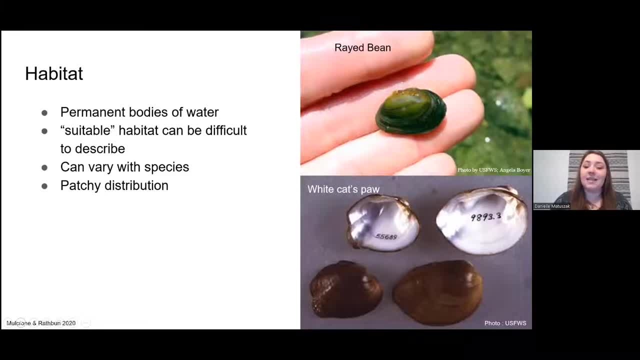 that kind of triangular shape, and so these two muscles are actually um endangered. they're threatened um because of, you know, habitat loss and many other threats that i'll get into a little bit later. a key thing to know about freshwater mussels is just because there's freshwater. 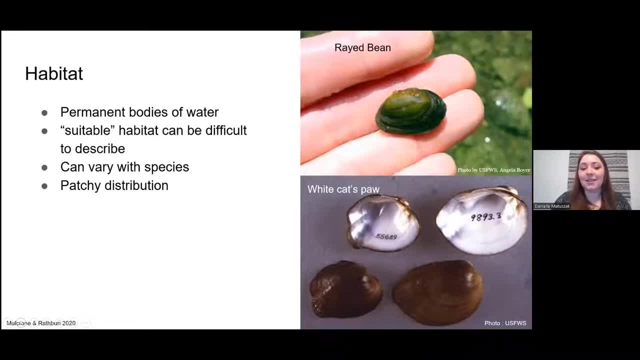 mussels in a stream or in a lake doesn't mean you'll be able to find them easily. they are kind of patchy in their distribution that specific areas within a lake or specific uh sections of a stream channel or sections of a streams course may not be suitable, though we 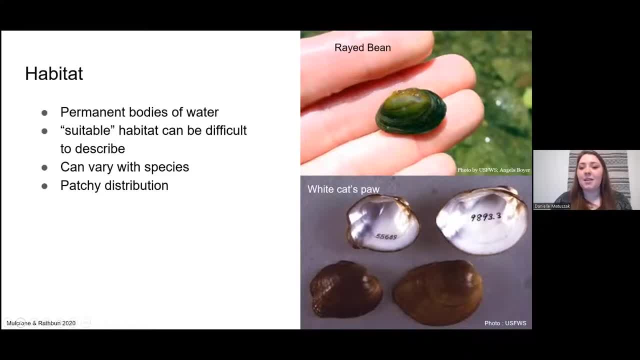 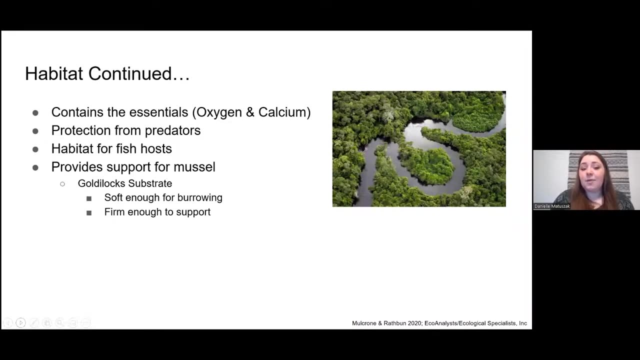 can't describe suitable very well for some species. they're patchy. they will go to a specific area or in a small subsection of that lake or stream. so surveying them, finding them, can sometimes be a little bit difficult. and with with habitat, the few things we do- kind of know. 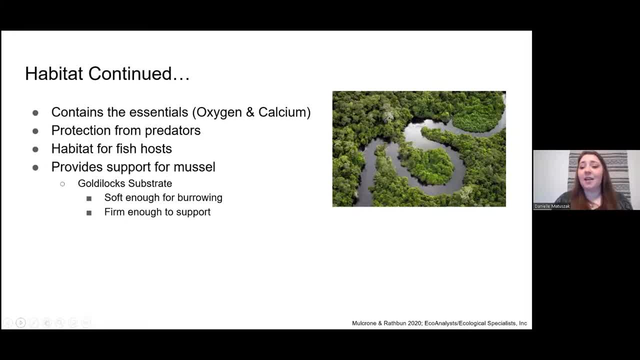 that we need for freshwater mussels to be successful in living in their habitat and maintaining populations is the water needs to contain and set the essentials: oxygen and calcium. so they need that calcium in order to build their shells- oxygen to survive, and so they also need protection from predators and also habitat for their fish host. i said that that, uh, fish. 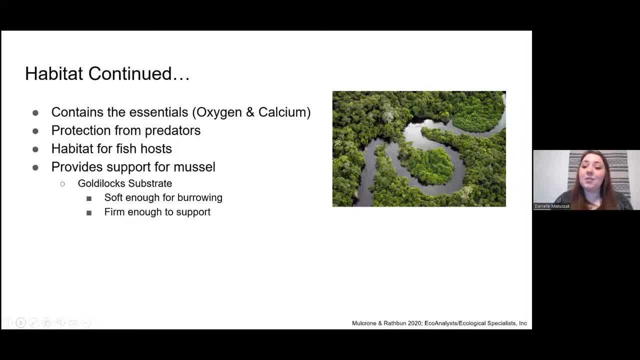 host would come back again. well, here it is again. if their fish hosts are not able to survive in a section of stream or in the lake, there's a good chance that the population of mussels that are there will eventually die out, since they aren't able to reproduce. 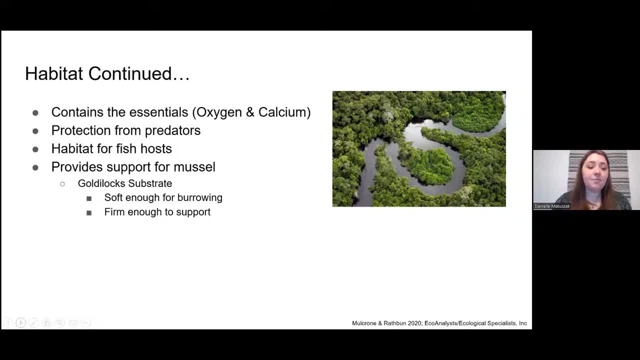 using those host fish with that parasitic phase. the other thing we need is support for the muscle in the form of the substrate, and so this is kind of the goldilocks, so it needs to be soft enough for burrowing but firm enough to support. so somewhere in the middle is kind of that goldilocks. 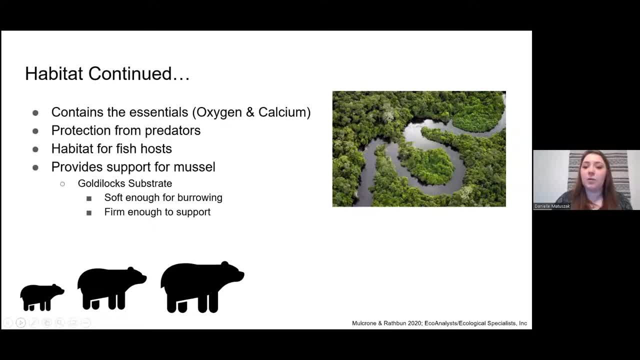 thing of the goldilocks and the three bears. so it's soft enough to burrow in and able to mature for those juveniles, but firm enough to support it that it doesn't sink in or kind of get lost in the muck in the bottom of a stream or a river. 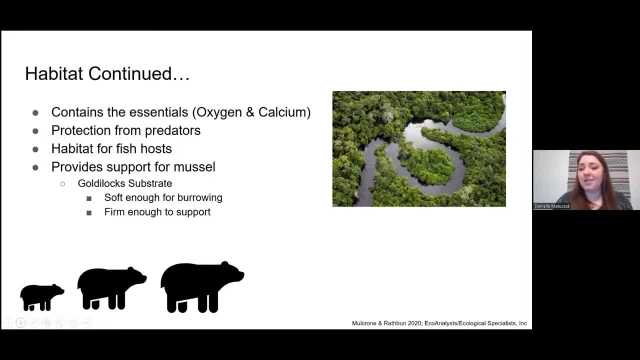 and these things go the same for, kind of, if you're in a stream system of not too fast of flow but not too slow flow of the water, not too deep but not too shallow. the goldilocks is very common when it comes to discussing muscle, heavy muscle habitat. 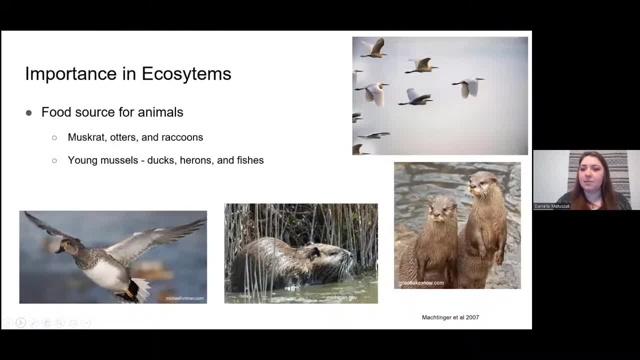 and so, as this title is talked, the importance of freshwater mussels ecosystems. in many ecosystems they serve as a food source for a wide variety of other organisms, both organisms that are terrestrial, some that are both aquatic and terrestrial, and you know just aquatic organisms, so muskrats and otters and raccoons. they will all feed on the adult. 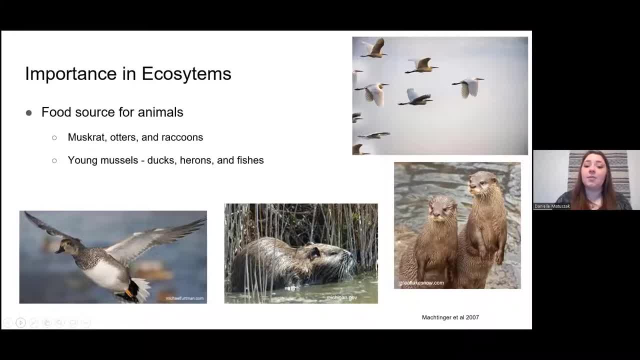 muscles, and sometimes the juveniles as well, whereas younger muscles are often predated upon by ducks, herons, many fishes, and so i have a couple of those organisms pictured here. on the bottom left we have ducks. in the middle there we have a little muskrat, of which i have one living behind. 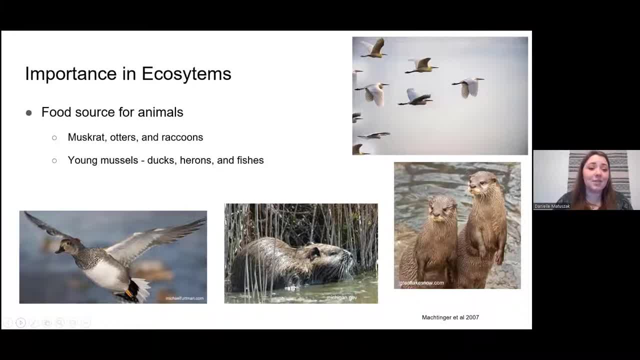 my apartment, so i've seen it in the water and along the edges of the kind of pond that i have in my backyard, and then there's also otters, and then also herons, and there's a variety of other organisms that also utilize muscles of all different species as a food source. 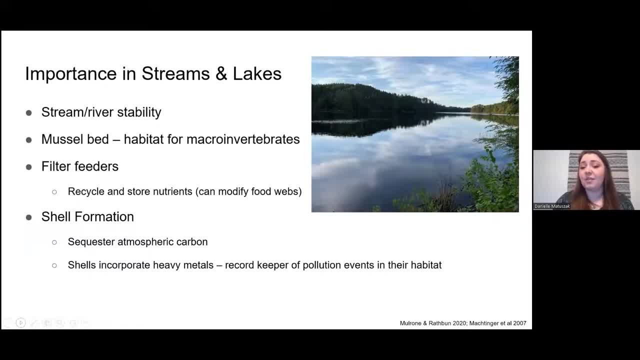 additionally, they're very important for stream, river stream and river stability. muscle beds often provide a habitat for macroinvertebrates. when i say macroinvertebrates, i'm talking about either crayfish, something that doesn't have a vertebrate spine, with looking at, you know larval stages of potentially terrestrial insects. 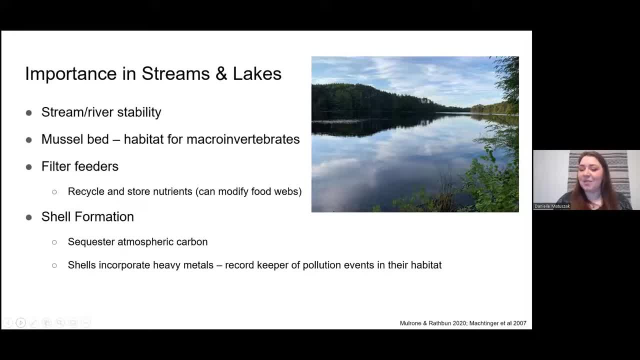 or aquatic insects, but muscle beds make excellent hiding places to help those macroinvertebrates avoid predation by fish of ducks. other type of organisms that would like to use them as their snack or lunch is that mussels are filter feeders In order for them to eat their lunch. 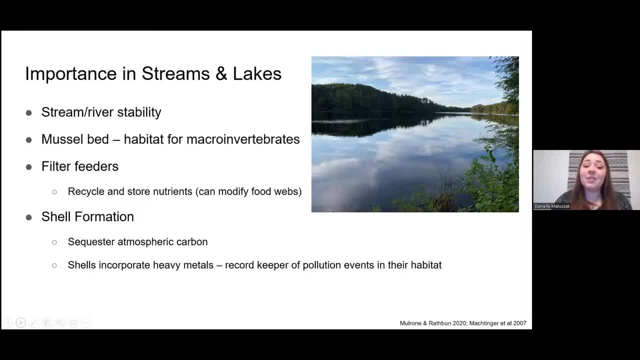 they will suck in water from the water body that they are in, filter it for the nutrients and the food that they want, and then put the water back out into their environment, And so they can recycle and store nutrients, which in many cases, can modify food webs. 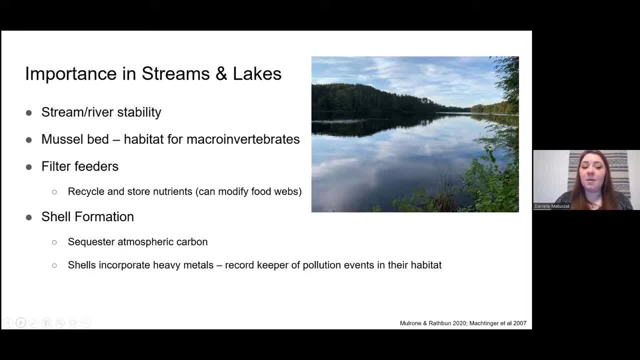 And I'll touch on it a little bit later when I talk about the invasive zebra mussels. but filter feeding is great, But when it comes from an invasive species it can be extremely detrimental. But these native mussels are able to help. 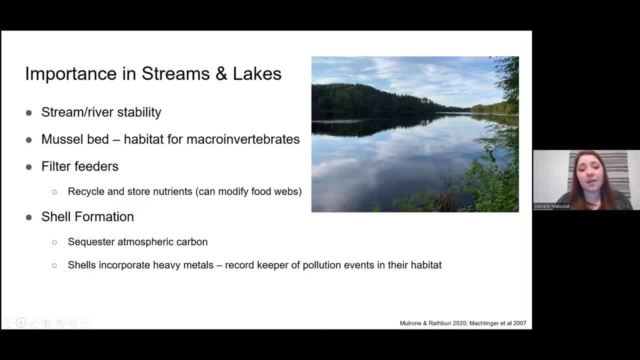 keep food webs stable, modify them to create a healthier lake or stream ecosystem, and those kinds of things. Additionally, there's shell formation. The interesting thing is that they can sequester atmospheric carbon, So some of you may know that there is an abundance. 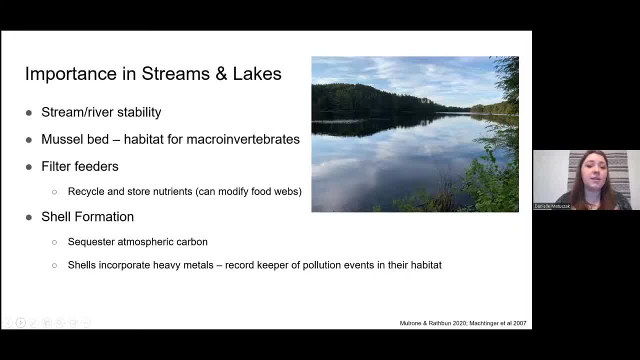 of atmospheric carbon now from the burning fossil fuels, many other things, And so these shells are able to sequester that. you know the natural, you know atmospheric carbon. So these freshwater mussel species are key to helping to kind of reduce the amount of atmospheric carbon we have. 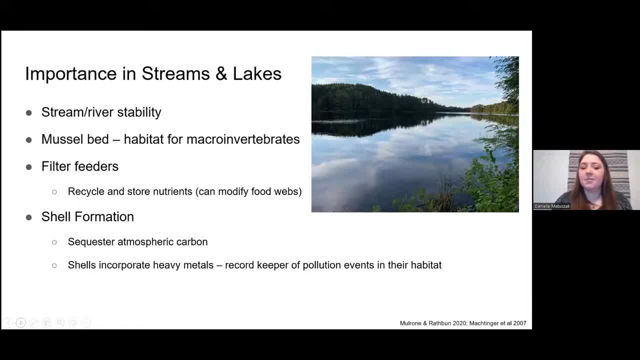 And additionally, shells can incorporate heavy metals. So when there's a large pollution event, or even a small one in their ecosystem, in a lake or in a river, creek, stream, they serve as a record keeper. You're able to tell when there was a large pollution event. 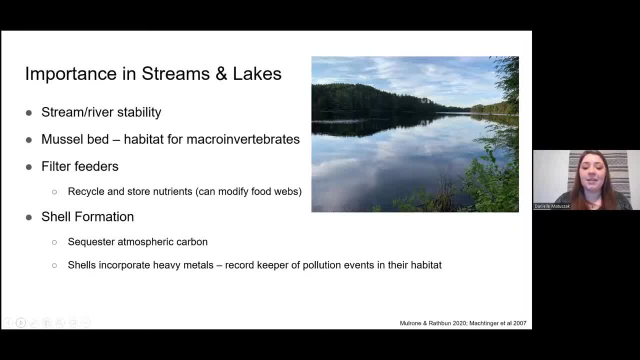 because you'll be able to see it in evidence in their shells, And so they'll be able to say: you'll be able to determine when a pollution event happened in their habitat based on that, since they do incorporate those heavy metals into their shells. 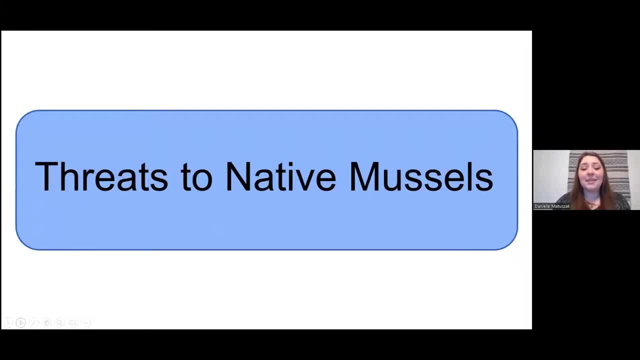 So I'm going to move into the threats to native mussels. Unfortunately, native mussels are quite threatened and there's a lot of things that we need to keep in mind when we're doing conservation, But when it comes to the threats to native mussels, 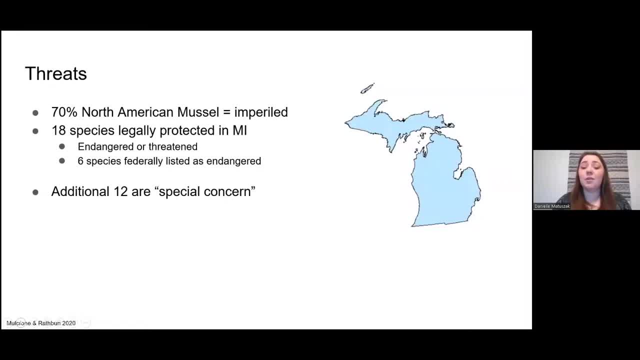 almost 70% of North American mussels are imperiled or endangered, And that's a lot, especially if you remember back to that introductory slide that North America is home to over a third of the worldwide population of species for freshwater mussels. 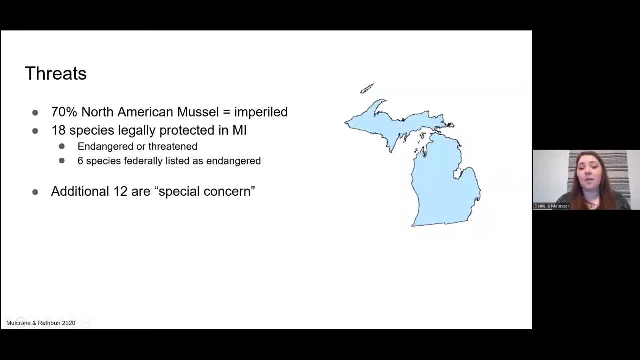 So if 70% of North American mussels are imperiled, that's a lot amount, a lot of freshwater mussel species that are not stable, aren't reproducing, not having enough habitat, all of those things, And so within Michigan, 18 species are legally protected. 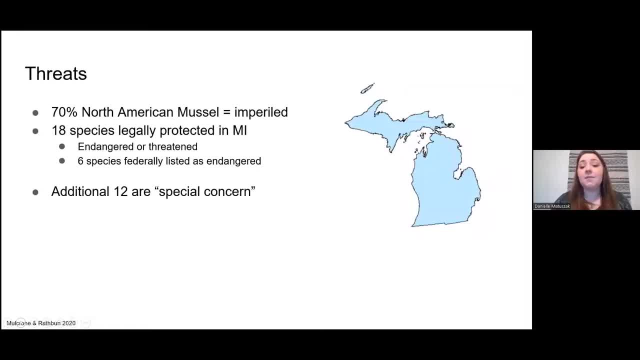 That are either endangered or threatened, And six of those species are federally listed as endangered and have federal protections against them or for them, And so an additional 12 species are listed as a special concern, And so I'll reiterate again, 70% is extremely large amount. 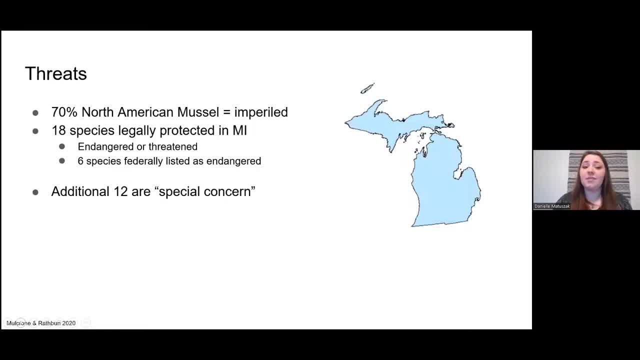 for there to be imperiled mussels, which is why conservation of mussels and sharing with the public, like all of you, about mussels and their importance is crucial for their conservation. One thing that you may not know is that mussels make money. 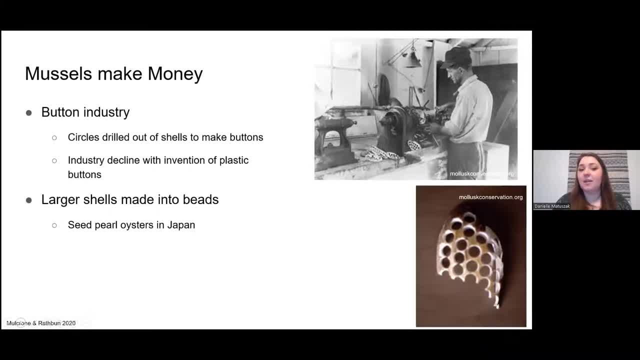 in more than one way, And so one of the first things that I'll talk about is the button industry. And so back in the 1800s, early 1900s, circles are drilled out of the shells to make buttons. People would go in and collect large amounts of mussels. 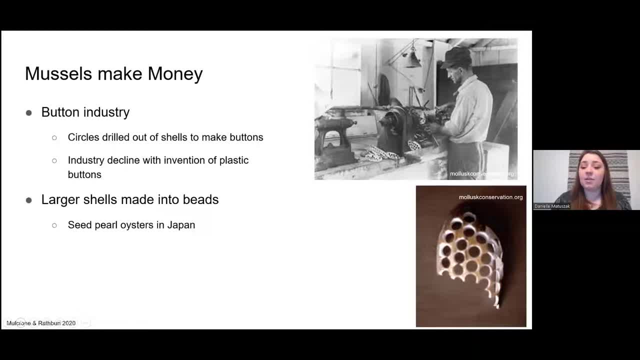 And some of you may see that in the previous picture that I showed where I had that white cat's paw, the inside of the mussel is that pearly white, shiny, beautiful inside, And so that was used to make buttons On the picture on the bottom right here. 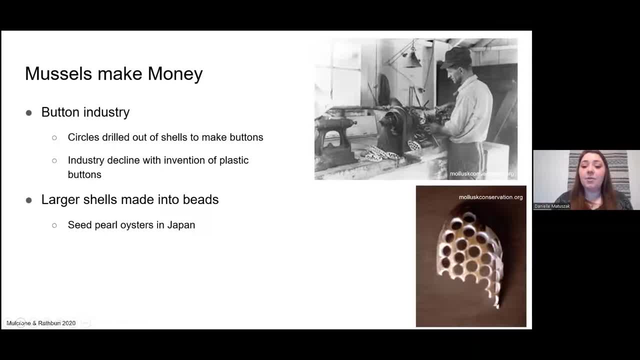 you can see how there's holes drilled out of these shells, and they would use those muscles to create buttons, And you can see in the upper picture there of the kind of drill dremel that they use to punch them out. And so eventually, this industry did decline. 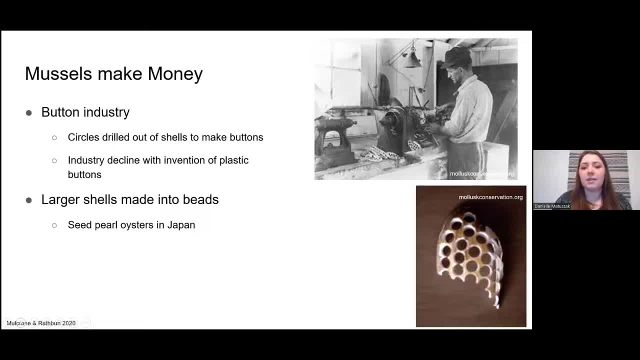 in the mid 1900s- about 1940s, 1950s, with the invention of plastic buttons. However, in many areas in the United States and the Midwest you can still find shells like the one pictured on the bottom right there that have holes in them. 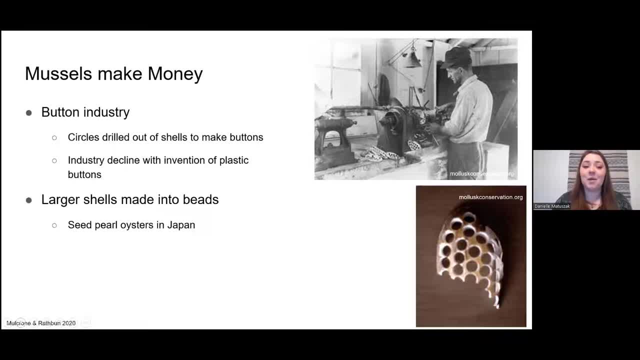 from when button making was utilized, primarily freshwater mussels, Additionally larger shells. larger freshwater mussel shells were made into beads, And so these were shipped to Japan to be used to seed pearl oysters. And for those of you that don't know, 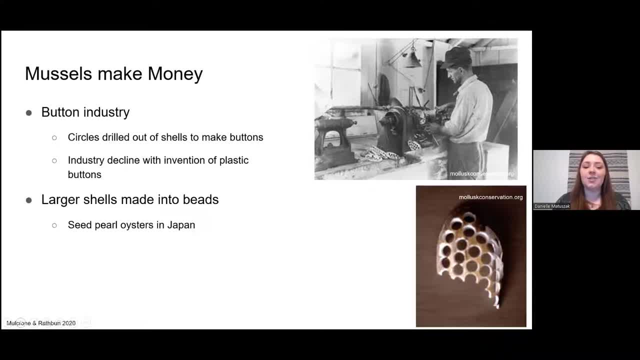 pearl oysters are oysters that create pearls for the kind of international pearl trade, And so many times they will need to seed a pearl oyster in order for it to create pearls. The way that pearls form is some sort of foreign body is introduced either naturally or, in this case, by humans. 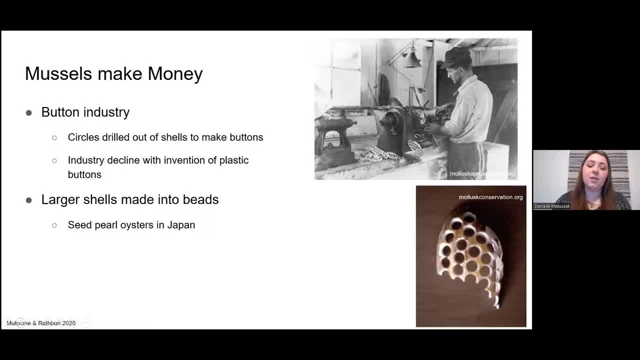 into the inside of an oyster And then the oyster, to protect itself, will put layers and layers around that foreign body, creating that pearl that we now wear as jewelry and that we see as kind of a fine, almost gemstone, of a way kind of a saltwater gemstone. 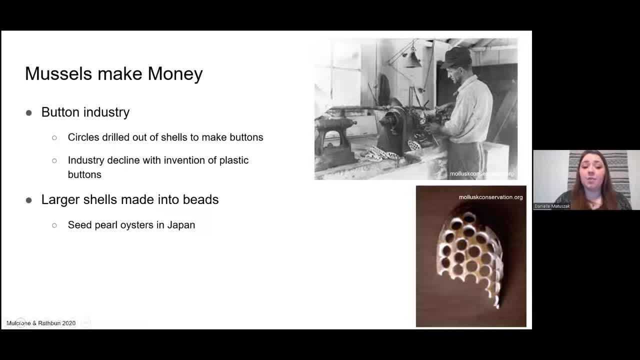 And so a lot of the larger shells those beads are made from them, shipped off and used as seeds for pearl oysters to create pearls to help foster that pearl trade. But unfortunately the combination of the button industry and then also the seeded pearl oyster 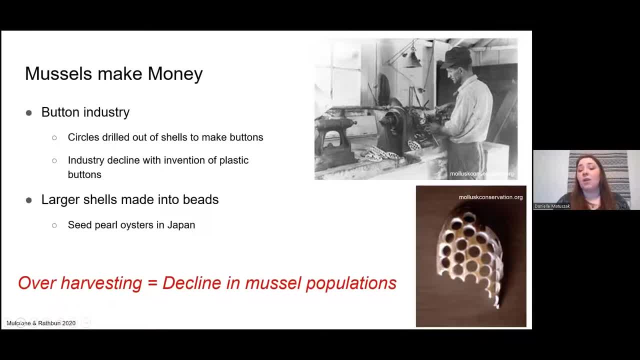 industry led to an abundance of over-harvesting, not only in Michigan but throughout North America, which led to a decline in mussel populations that we still see, But unfortunately this decline in mussel populations wasn't really noticed or registered. until the 1970s, which is really unfortunate, since they had been over-harvested for decades, almost a hundred years at that point. And another threat to them besides the button making and being used as seeds for pearl oysters. 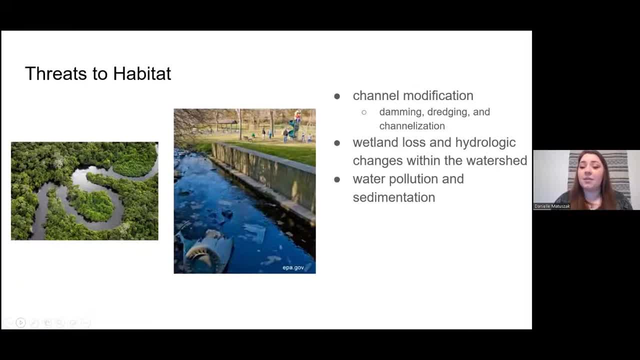 is their threats to habitat, And so my personal thesis research discusses dams and impoundments and reservoirs and how that impacts the spread of invasive species. And so my personal thesis research discusses dams and impoundments and reservoirs and how that impacts the spread of invasive species. 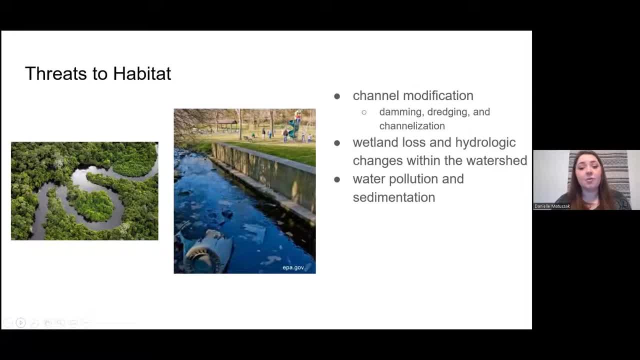 And so my personal thesis. research discusses dams and impoundments and how that impacts the spread of invasive species, But channel modification by damming, dredging, channelization can be very detrimental to freshwater mussel populations by changing their habitat or, in a lot of cases, completely removing the habitat. 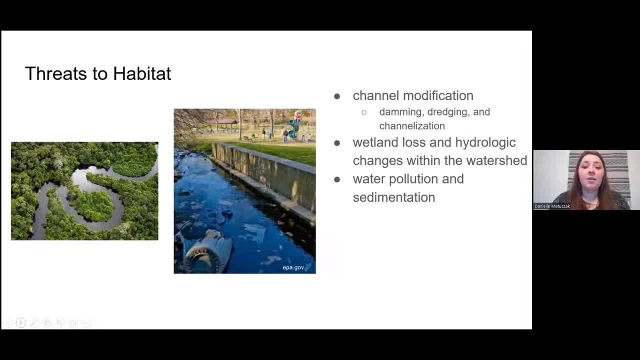 they would need in order to have a healthy population. I have to show a picture here on the right that shows from the EPA a stream bank that has had a retaining wall put against it, And so this basically eliminates part of the stream bank. 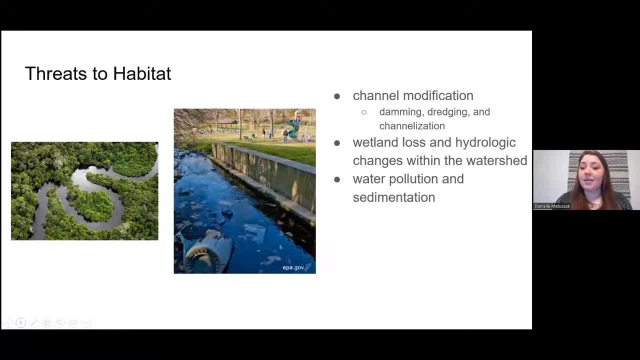 And so this basically eliminates part of the stream bank, A stream bank that would lead into the water and that may have been home to freshwater mussels. But now that there's that retaining wall, that habitat has been changed, likely permanently, And so it may no longer be suitable. 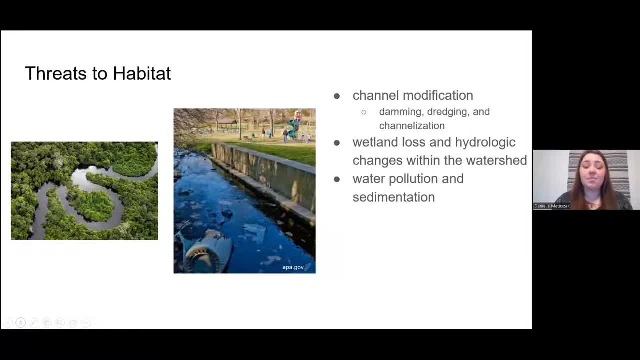 for those freshwater mussels, Wetland loss and hydraulic changes for the watershed, So altering of flow regimes, drainage of wetlands, many of those other things, Since those that you don't know. wetlands are very, very important to being water purifiers and cleaning the water. 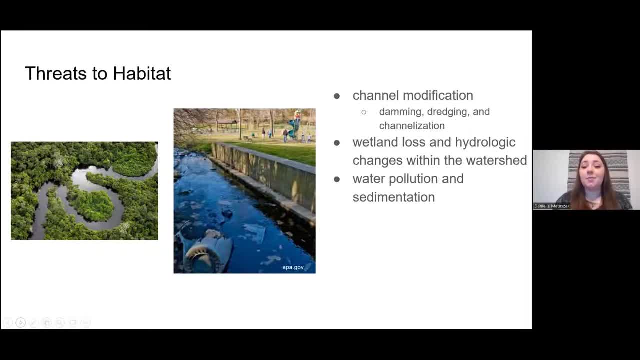 before it gets into streams and lakes. So wetland loss can lead to higher water pollution and sedimentation, And so in the picture I show here it is quite an urban street or a stream, but you see that there's pollution in there, and pollution and sedimentation are quite detrimental. 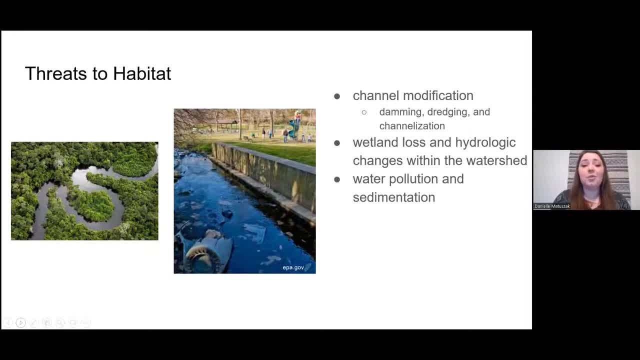 to those freshwater mussels Just in general, from the pollution from toxins, chemicals that can hurt or kill freshwater mussels, or sedimentation that can cause it difficult for them to filter, feed or bury them, all of which again hurt and are threats to those freshwater mussels. 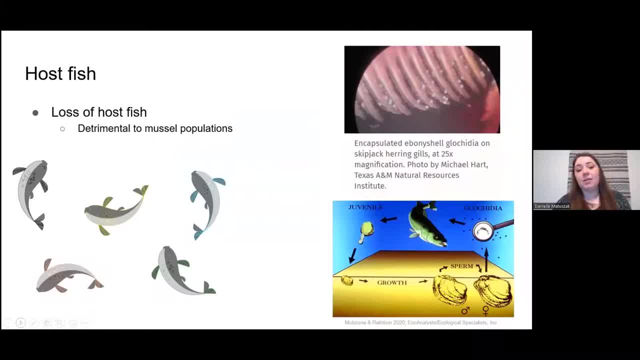 And I told you once again that it would come back again- is the host fish. When we're building dams or removing dams and we are altering flow regimes, altering the courses of rivers and streams and lake connections, a lot of times, while we may not directly be impacting an actual mussel, 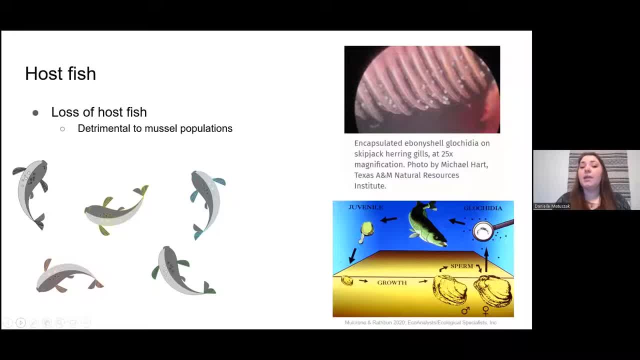 you're not physically moving or killing a mussel. you're removing the habitat that's needed for host fish And, like I said, mussel populations are reliant upon the populations of their host fish. So if you lose the habitat that your host fish needs, 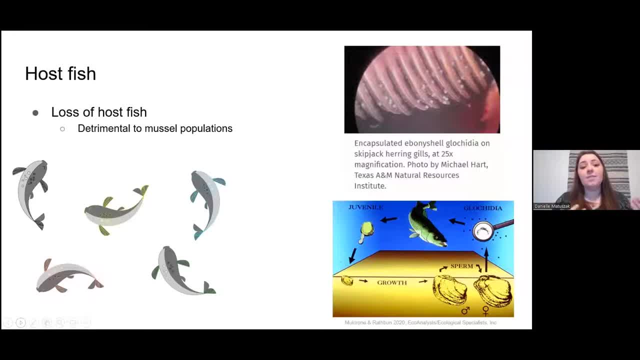 to survive and reproduce and keep a healthy population for fish, it's gonna be detrimental to mussel populations. And so if you're sampling for mussels and you see that, oh, there's still population of this freshwater mussel in this stream, but they're all adults. 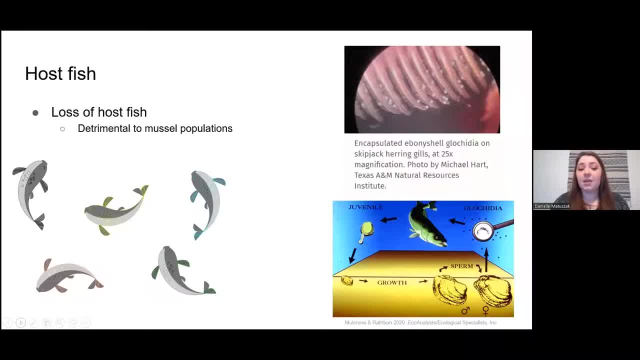 and you don't see any juveniles, this may be indication that the host fish is no longer there, And so, yes, there's adults there, but they're not able to reproduce and to continue to build that population. replace the mussels that die off. 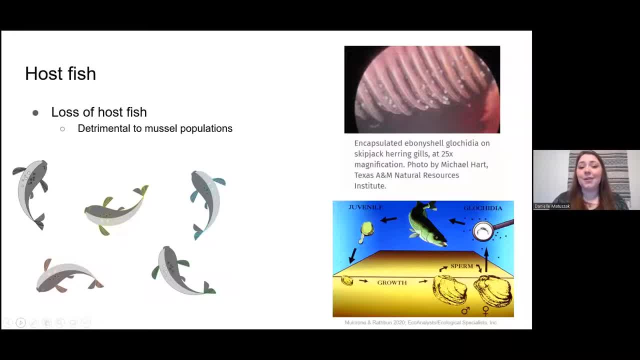 and to create a larger population. So again, host fish are extremely critical, And so I included the life cycle from the previous slides, but also on the upper right-hand corner there you see that. that is just a quick image of what it looks like for those broccidia to be on the gills. 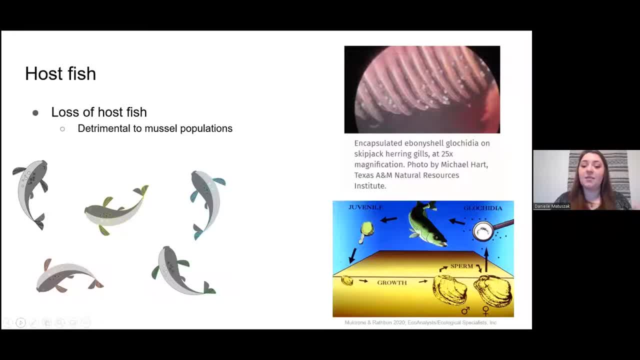 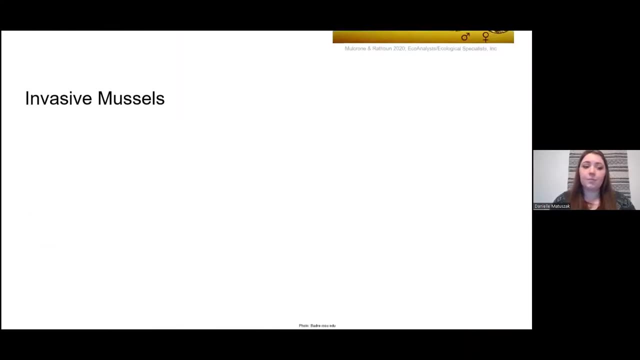 And so they're in there, stay there until they become juvenile mussels and then fall off again. To reiterate, host fish extremely important to not only the biodiversity of freshwater mussels but just for the sustaining of their populations. And so I mentioned 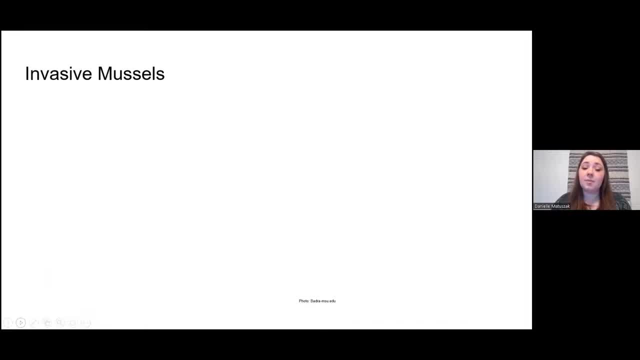 that there are three different invasive mussels. My research focuses on the invasive zebra mussel, but these are three different invasive mussels that are in Michigan and in parts of North America. The first is the Asian clam, which is pictured down here on the left. 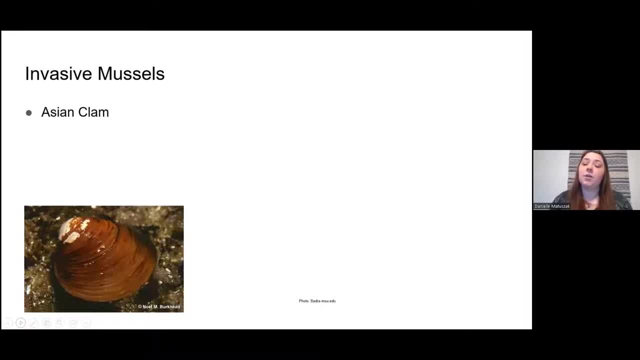 kind of a circular clam round, And so these are invasive. They're related to, they're very similar and related to a native version, but these are specifically invasive. Then we have the zebra mussel: Dracaena polymorpha. 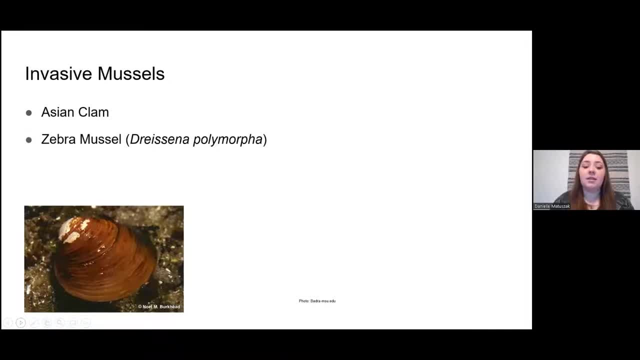 which is a scientific name, which is what my research focuses on, And they look like this. However, it is not the large mussel that you see, rather all those little zebra looking mussels with those zebra looking markings on them that have attached themselves to this adult mussel. 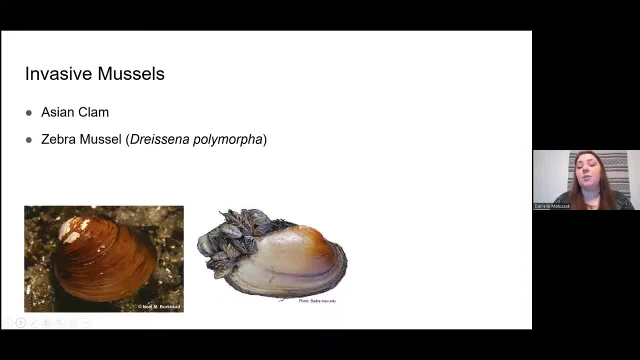 That's the zebra mussel, And this is one of the reasons why they're quite detrimental to freshwater populations. And thirdly, a close relative to the zebra mussel is the quagga mussel, And so we can see that here. 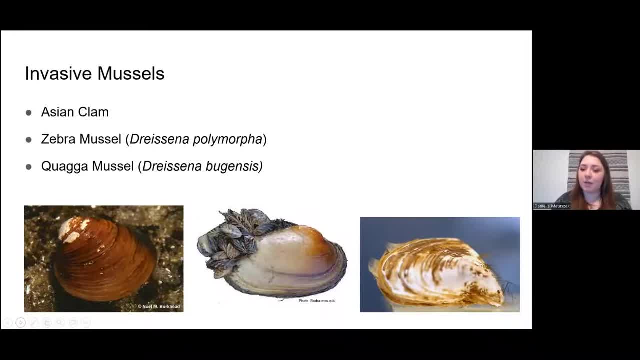 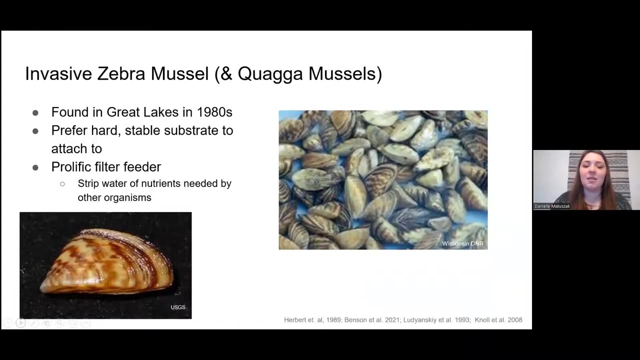 they're fairly similar in size and shape in general, and are also extremely prolific filter feeders, similar to their zebra mussel friends, And so since my research is about invasive zebra mussel, I couldn't resist putting a slide in about them. 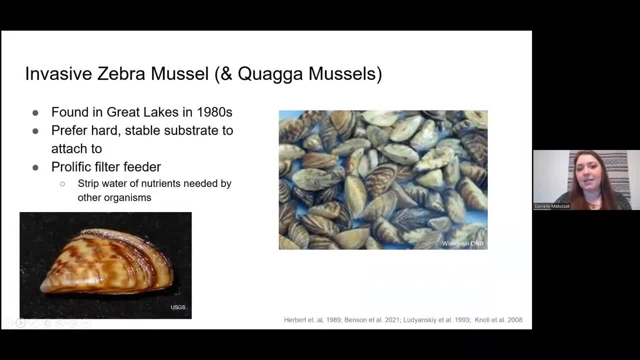 And so the invasive zebra mussel was found in the Great Lakes in the 1980s. It's thought that it was brought to the Great Lakes through ballast water, through the shipping trade, when the canal system through the Great Lakes 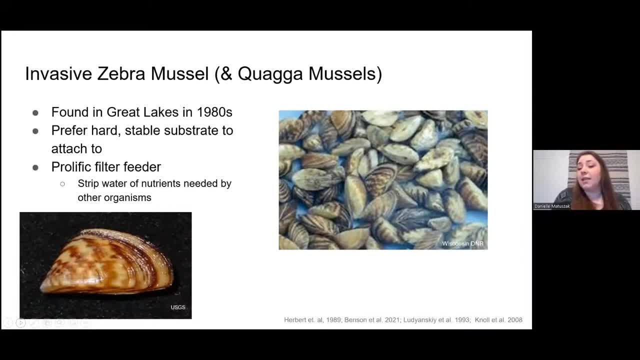 but there is evidence that they were potentially in the Great Lakes earlier than the 1980s. but it is the well-acknowledged that the 1980s is when they were firmly established And so invasive zebra mussels prefer hard. 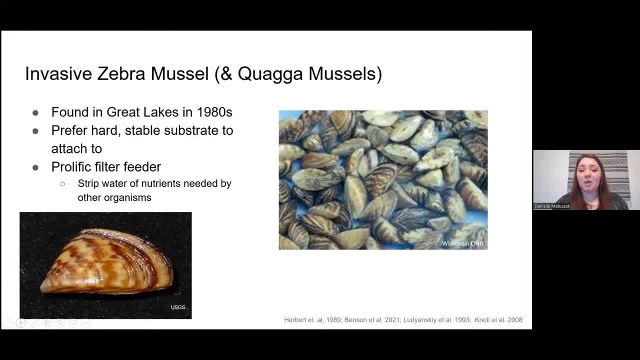 stable substrate to attach to. Well, something that is hard and stable is existing freshwater mussels, as is that picture that I showed on the previous slide. They will often attach to freshwater mussels, either starving them by out filter, feeding them as the prolific filter feeder. bullet point there. 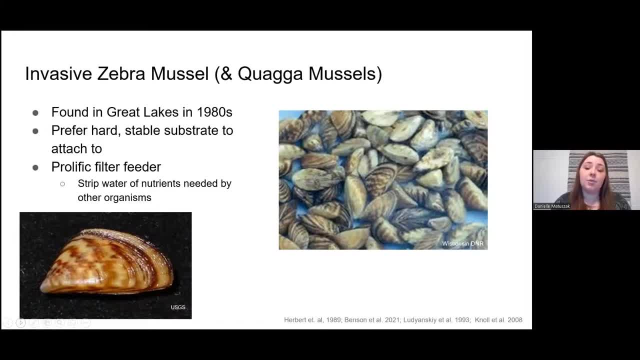 says, or they will create it so that they are not able to reproduce. since they're not able to open up, They're also not able to feed if they cannot open. So zebra mussel populations can basically stifle native species by attaching to them. 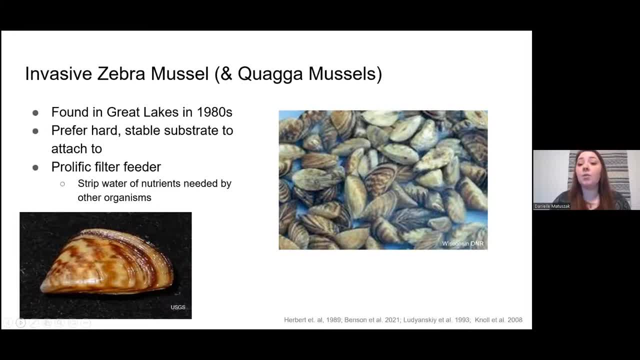 basically starving them by stripping the water of nutrients needed. for other organisms, including those freshwater mussels And quagga mussels, their close relationship has the same thing, being prolific filter feeders, and they're not able to feed themselves, So zebra mussels are also attached to native mussels. 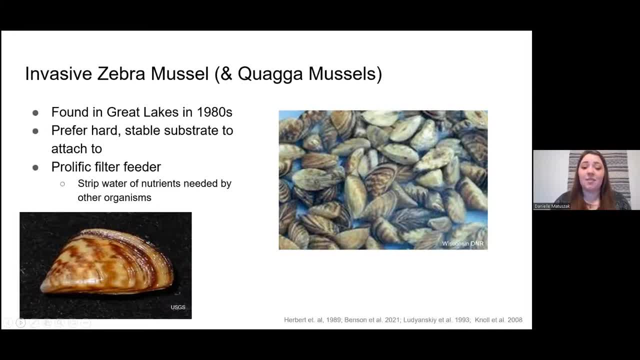 and are extremely detrimental to the native mussels. We've seen in the great lakes that after the introduction of zebra mussels into the great lakes, we saw the great lakes get extremely, extremely clear. Some people think that's great. It's actually stripping a lot of the nutrients. 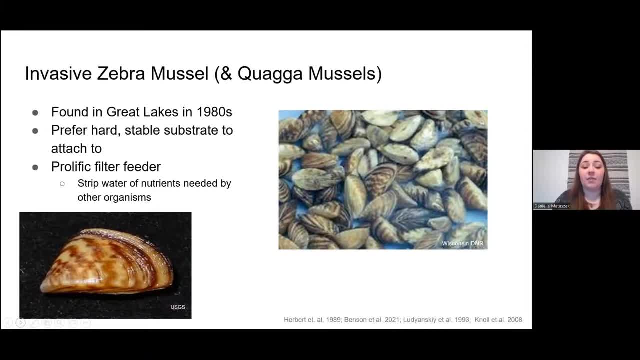 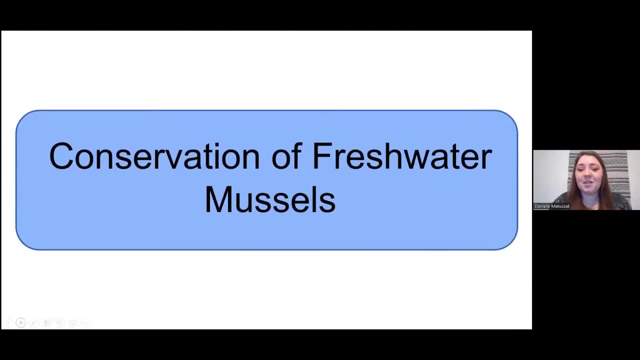 from the great lakes, creating it very difficult for other organisms to survive on what's left. And so, finally, something little less doom and gloom is the conservation of freshwater mussels, And the conservation of freshwater mussels has been slowly making improvements over the past years to not only 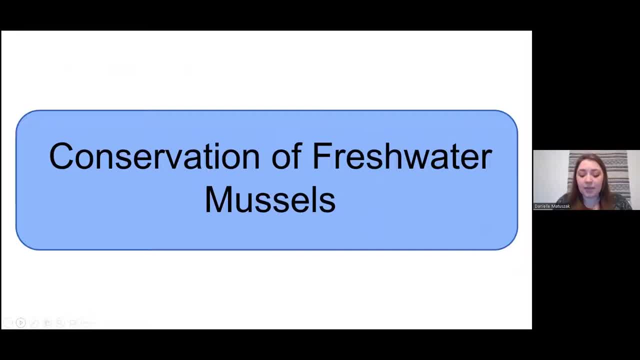 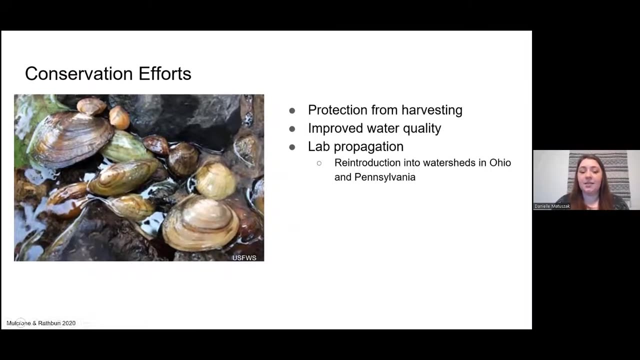 preserve existing freshwater mussels but also make sure that we're setting up foundations for future preservation and conservation of freshwater mussels, not only in Michigan but throughout the United States and North America. And a couple key things that I want to make note is that in Michigan there are protections for freshwater mussels from harvesting. 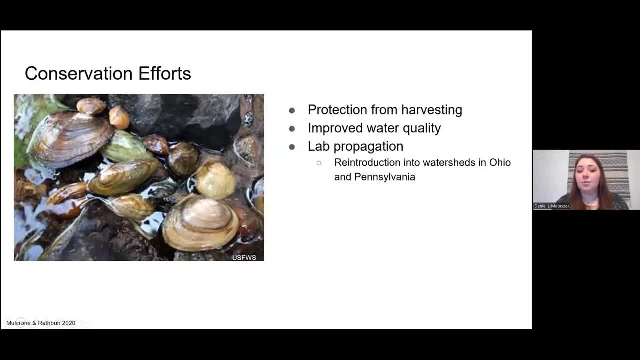 So, as you are out on your lakes, going through streams, creeks, it is very fine for you to pick them up, look at them. However, make sure you put them back down in the exact same spot, in the same way that you found them. It is illegal to harvest them and take them with you. though some harvesting. 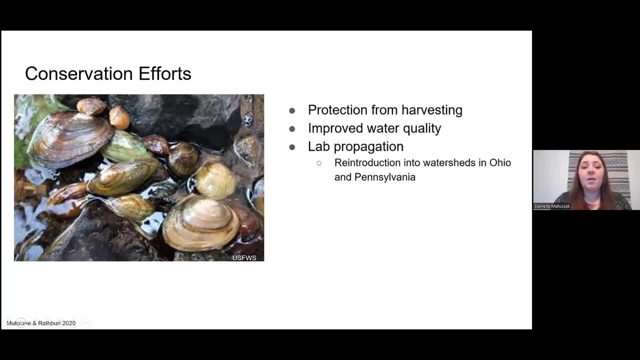 can be done if you apply for the correct permits, But conservation efforts have created the opportunity to do that, And so I want to make note that in Michigan there are protections for these, protections from harvesting to make sure that the mussels that are there are able to. 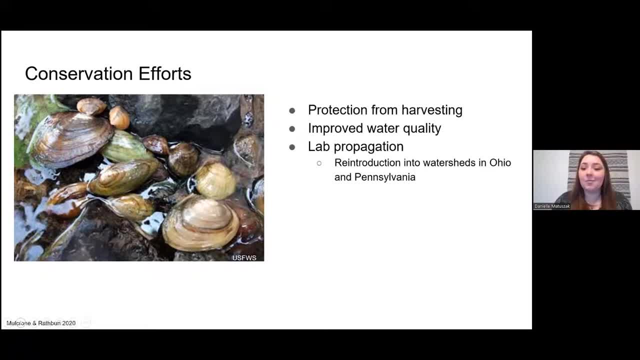 sustain the population, reproduce and so that we aren't losing a bunch of mussels from over harvesting, as we saw when we had the button trade, with the harvesting of mussels to create the buttons and for the seed pearls. Additionally, a lot of conservation efforts, though not focused. 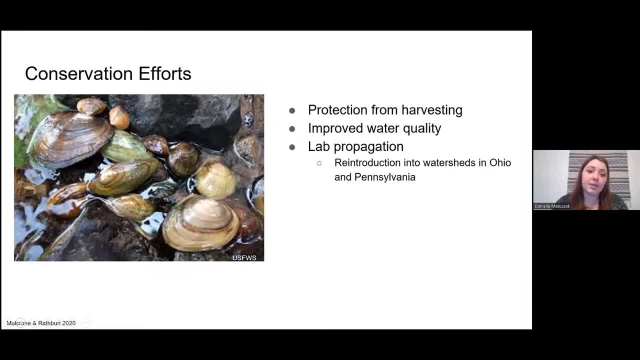 on freshwater mussels have been focused on improving the water quality of lakes and streams throughout the United States and in Michigan. This improves the water quality of the lakes and streams and it is extremely helpful for freshwater mussels. If we're improving water quality, we're 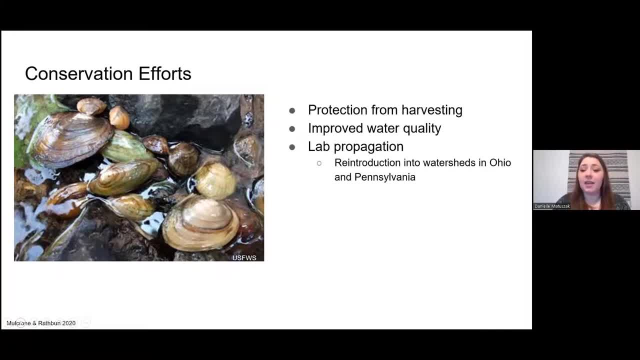 reducing the number of pollutants or reducing the eutrophication or the high nutrient loading in a lake or stream, which can help improve this water quality and help create healthy water for our freshwater mussels to be in. And then some exciting stuff is that lab propagation is proving to be. 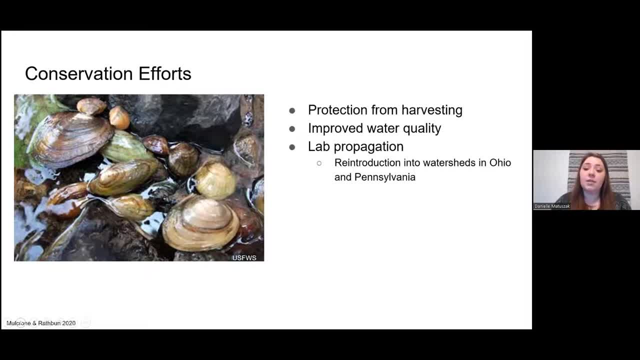 successful. There have been reintroductions into watersheds in Ohio and Pennsylvania of freshwater mussels that were originally there but had disappeared due to habitat loss, harvesting bad water quality, and so they were propagated in the lab and reintroduced into. 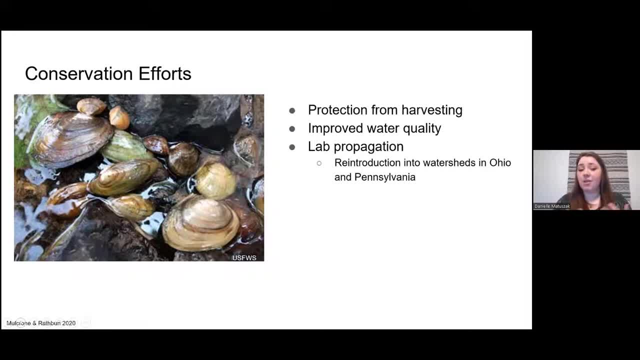 watersheds. This is extremely promising for Michigan and all over North America that in areas where there used to be freshwater mussel species but are no longer, if we're able to rebuild and restore that habitat, there's a chance that we're going to see that happen. So it's really important to 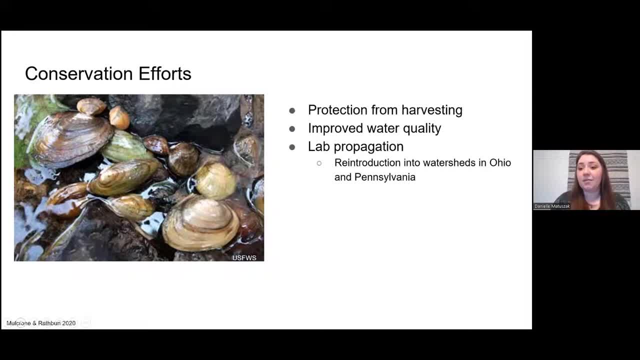 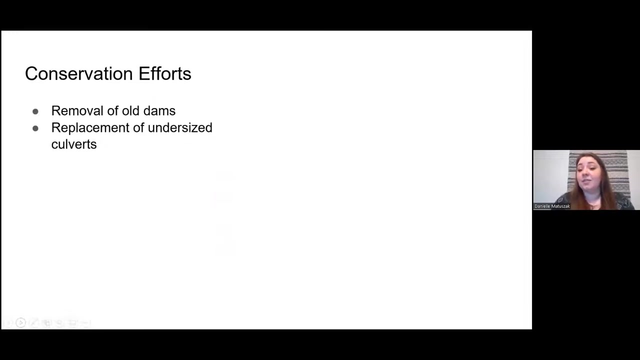 reintroduce these freshwater mussels back to their native ranges and help kind of boister and boost up that population of mussels which in turn can help boost water quality even more and help maintain healthy ecosystems in streams and lakes. The other thing is the removal of old dams and replacement of undersized culverts. So over the 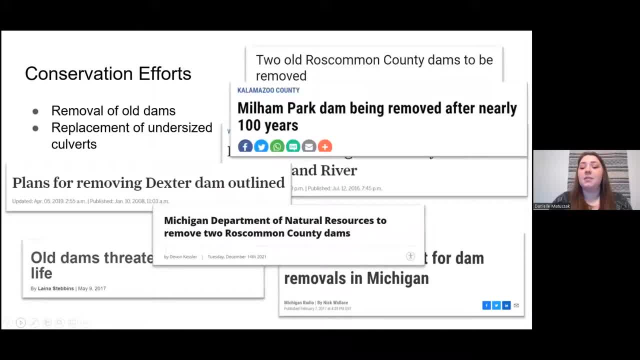 past many years, the removal of dams and replacement of undersized culverts has been an important part of what's happening in the United States. I believe about 90% of the dams in the United States are over 100 years old. It was back in the early 1900s when a lot of these were built. 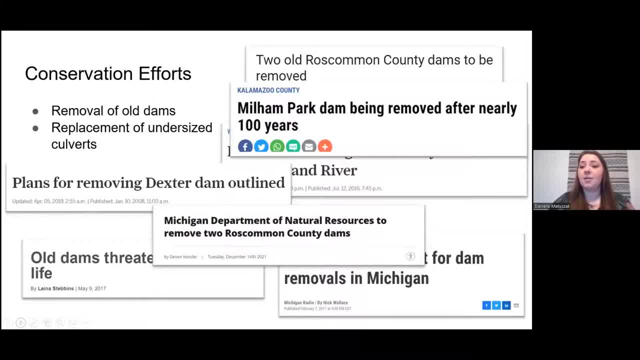 during the Great Depression, kind of boistering providing jobs to feed America, basically. Well, a lot of those dams are old and unstable, not safe, and so removal of these, while very good, has to be done carefully. So I think it's important to be aware of those dams. 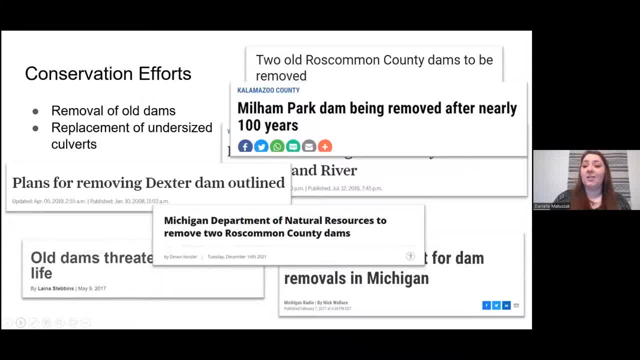 Taking into consideration that, while removing the dam can open up a previously unconnected, in a way stream system. you have to be careful when you're removing these so you're not introducing contaminants that were in those dams, making sure you're not creating too much sediment. 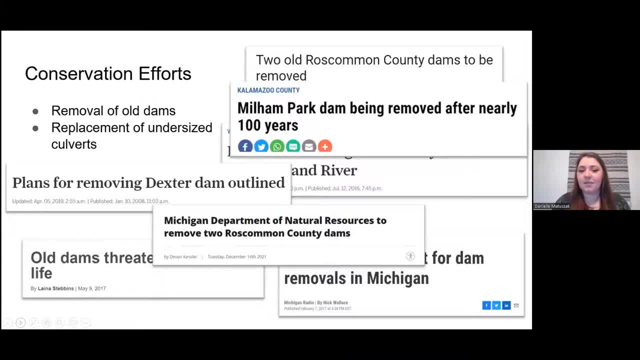 loading in the water for that sedimentation. that can hurt freshwater mussels. But when you remove those dams you're able to reconnect two sections of a river. You can reconnect lakes, which allows for those host fish. again it came back again. 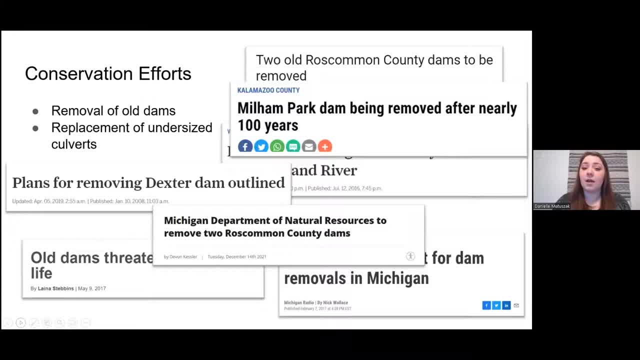 that reconnecting those water systems can allow the host fish to now go back and forth and to potentially have more habitat for them, which can lead to a higher population of freshwater mussels if they have that host fish that they need Additionally replacing undersized culverts. 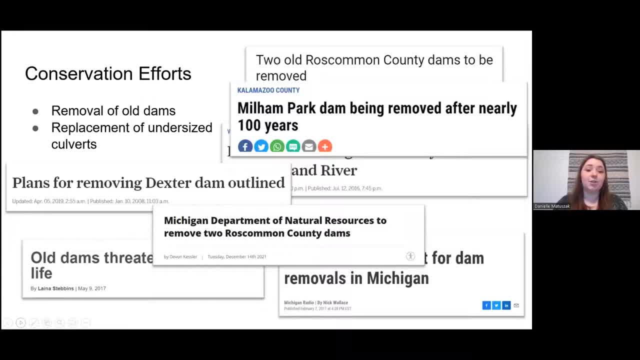 so when you have a road that is kind of breaking up a stream channel or a stream section, having a culvert that is too small, And by culvert- for those of you that don't know what it is, I didn't know that was the actual name for them- it's the tube that kind of goes underneath. 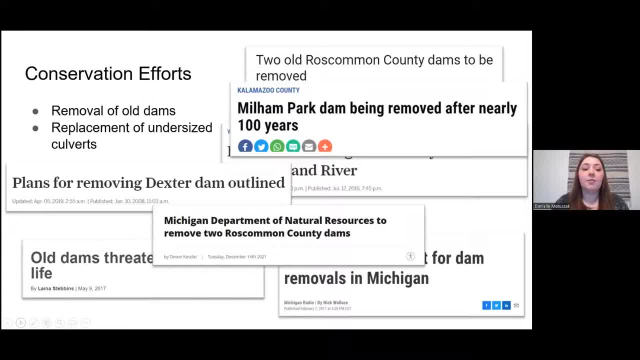 the road and it's the tube that kind of goes underneath the road and it's the tube that goes below the river and it takes a legal step to get back into that river And there are several different versions of it. But creating a larger culvert allows the fish to go through higher water. 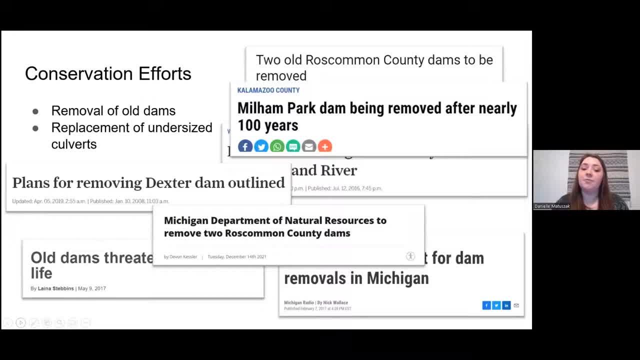 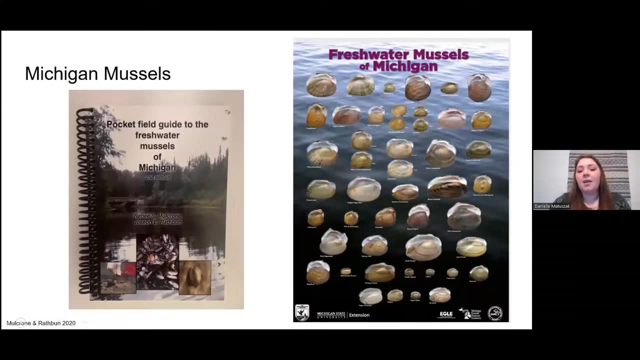 flow, again connecting that habitat so that the mussels and the freshwater fish that go with them are able to have habitat that's suitable for their reproduction and to sustain a healthy population. And finally, I want to do a quick kind of shout out to Rene Mulcrone and Joseph Rathburn and the Council of Fishermen for that wonderful job that they're doing at the Randolph Hope Preservation and the African Fish Conservation Society. And that is the entire team of the RANDOLPH HOPE Institute is working on. the entire team of the RANDOLPH HOPE Institute is working on. the entire team of the RANDOLPH HOPE Institute is. 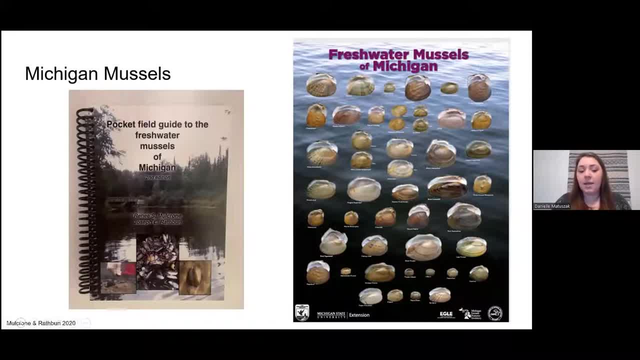 Joseph Rathburn and their Pocket Field Guide to Freshwater Mussels. It is an excellent resource for Michigan mussels and was used as partially the basis for this presentation and this talk, And so, in this kind of pocket field guide, illustrates a lot of the identification for. 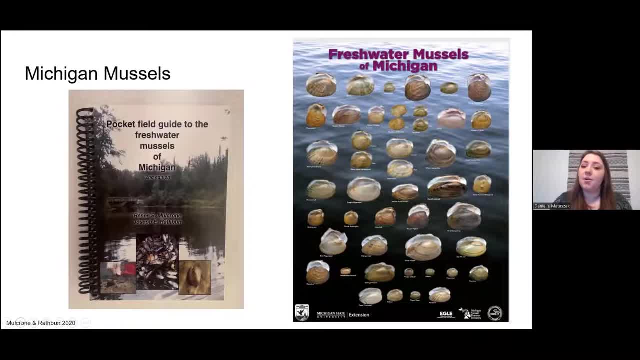 native mussels in Michigan, as well as a lot of the background that I went over in the beginning of my slides, And Michigan mussels- all 43 of them- are extremely important for our ecosystems and for lakes and streams and all of the aquatic systems that we have, not only in Michigan, but 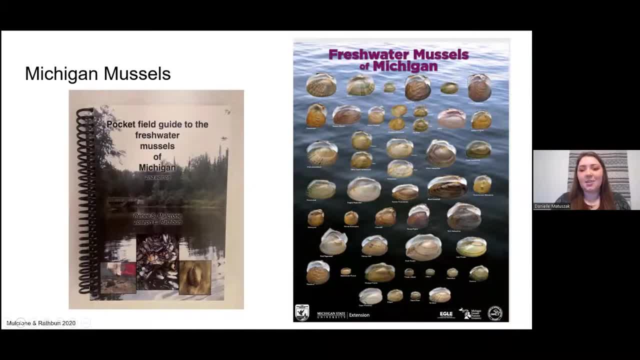 in North America and around the world, And it's extremely important to make sure that we're keeping freshwater mussels, even though they're very well hidden sometimes with their patchy distribution. keep them in mind as we're doing freshwater conservation work and sampling, and 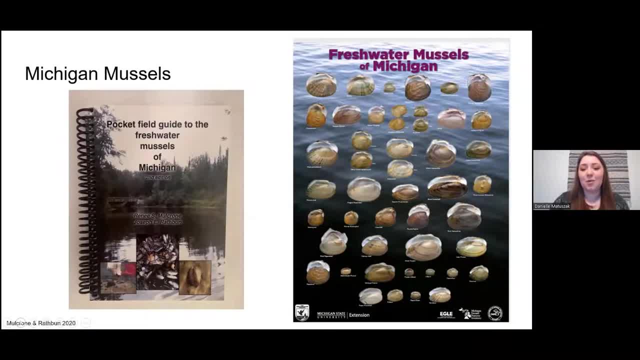 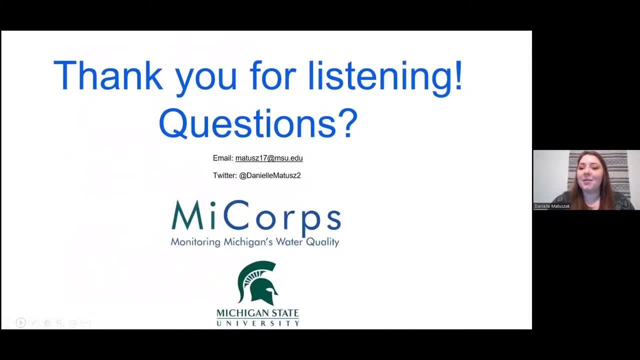 all of these other things that we're doing, And so I'm going to turn it over to you and I'll see you in a minute, And with that I want to thank you all for listening. I thoroughly enjoyed discussing freshwater mussels with you guys, and I'm very much open to any questions. My contact information: 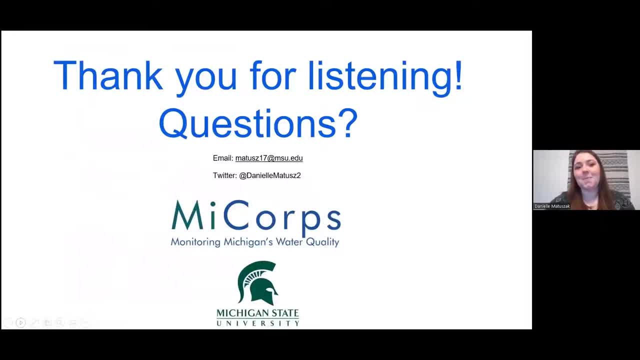 is also listed here if you think of something after the fact. Thank you, All right. Thank you so much, Danielle. I just put in the chat a link. if you're interested in that cool mussel poster that you showed, If folks wanted to get one of them for their own home or cottage, you can find one there. 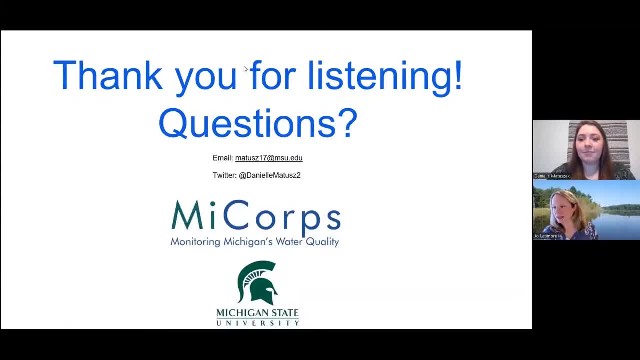 I did turn the chat back on here in a sec We're going to turn that on, But if you have questions, please put them in the Q&A box. I've had a few come in, So if you have any questions, I think without further ado, I'm going to pose a few questions to Danielle. 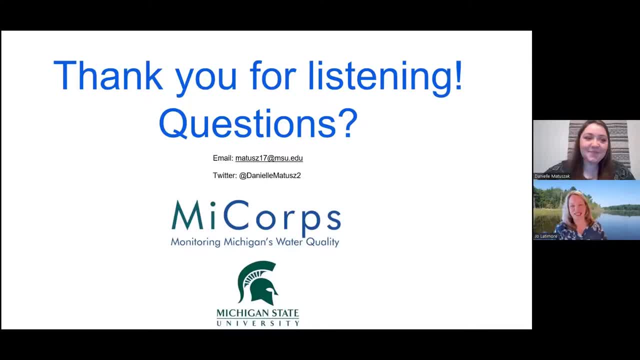 when she has a drink of water and gets her voice because she's been talking for a while. All right, So here's a two-part question from one of our listeners. One, how can you tell the difference between a zebra and a quagga mussel? And two, what is the difference between a clam? 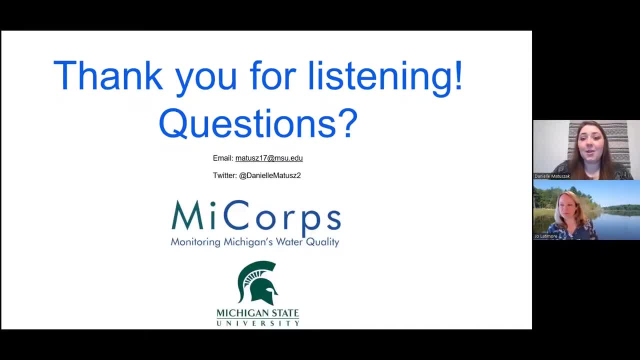 and a mussel, Or is there one? So for that first question- difference between a zebra mussel and a quagga mussel- let me see if I can go back to the pictures that I had of them, Back a few slides. 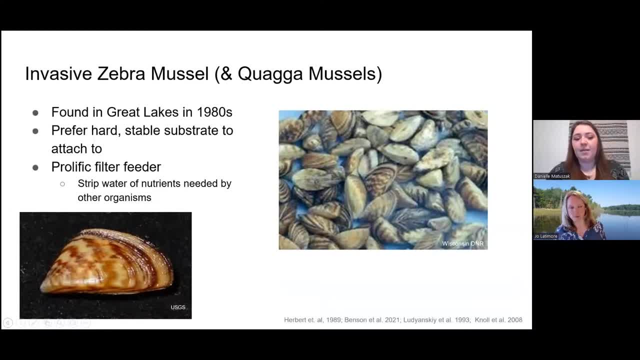 So zebra mussels, as you can see on the images here, have that kind of zigzaggy image kind of pattern on them, And that's one of the identifying things for zebra versus quagga mussels. Quagga mussels also have stripes on them, but they're much, much less distinct So they're not as 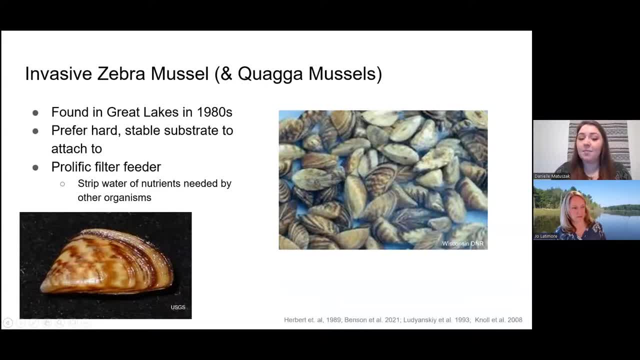 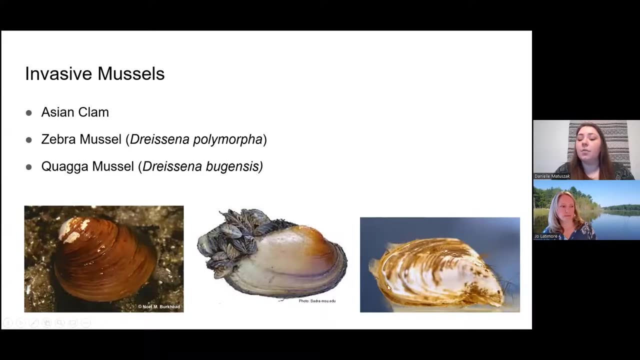 distinctive, And that is the way I learned how to identify them. As well. as zebra mussels are much more, as you can see here, kind of that very sharp triangular shape with that one flat edge. Quagga mussels are similar, However, they're a little bit more rounded and their markings are. 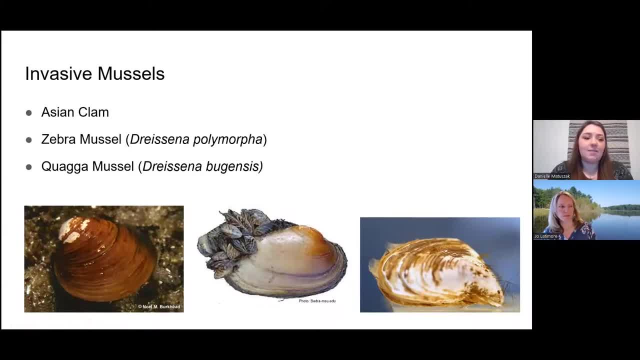 much less zebra-like, So that's kind of the way I would describe that. As for the second question, which I believe was the clams versus mussels, biologically I'm not too certain whether there's a specific difference When I was an undergrad. 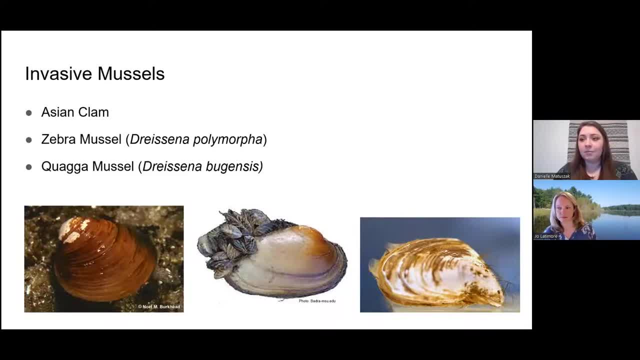 I used clam, bivalve mussel, mollusk, all of those interchangeably through common language, of just discussing it Scientifically. I believe clams are typically marine or saltwater organisms And mollusks can be freshwater or marine. So the zebra mussel. 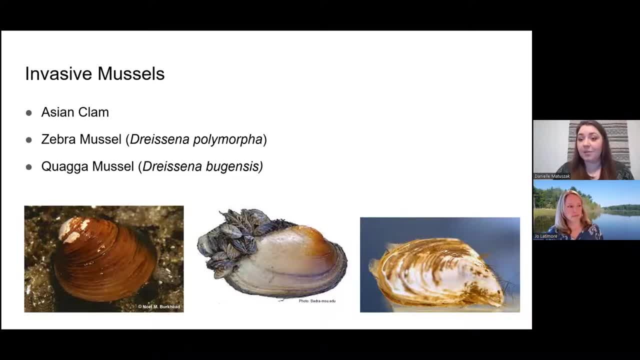 is originally from Eurasia, is able to survive in both marine environments as well as freshwater environments, So it's a mussel and it's found in both areas. I hope that answers that question a little bit. Great Thanks, Danielle. Another question that came in from one of our stream. 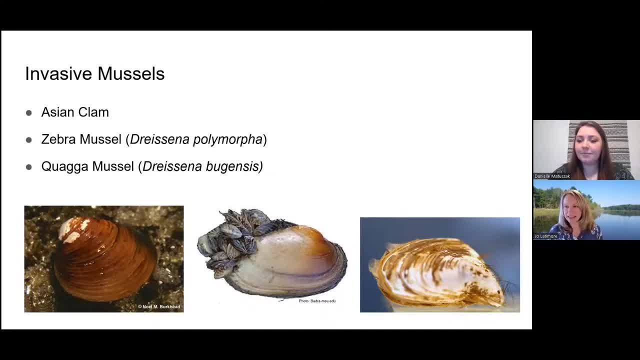 monitoring volunteers who's active in the MICOR program And they described how they collect invertebrates from the stream bed using a net and kicking around on the beach- So that's the stream bottom- And sometimes they get mussels in their nets. What should they do if they end up? 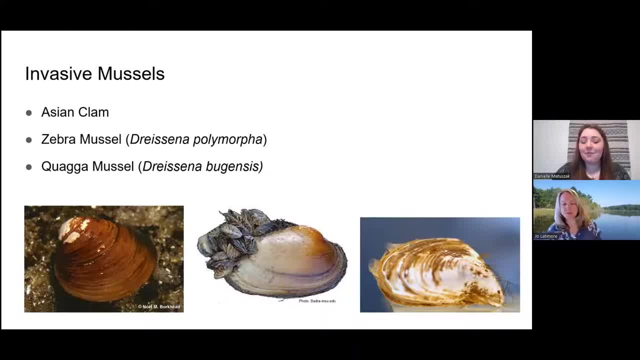 with mussels in their nets, Yeah, So first thing I would recommend is take a picture of it. Maybe you can identify it later on and that might help be able to identify what kind of mussels are in the streams that you're sampling. But the main thing is to make sure that you put that mussel. 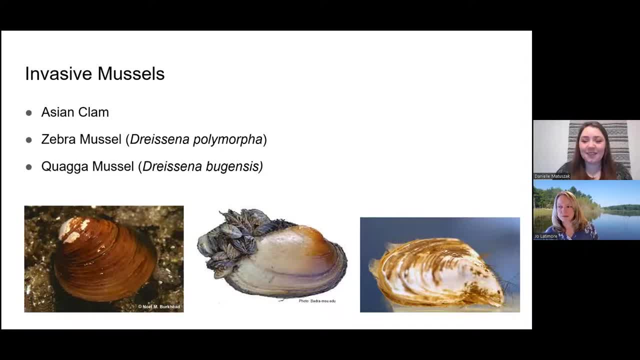 back in the water. Don't leave it out, Don't take it with you. The other thing is to try to kind of nestle it into the dirt, or not dirt but substrate a little bit, with the kind of hinge side as a way. 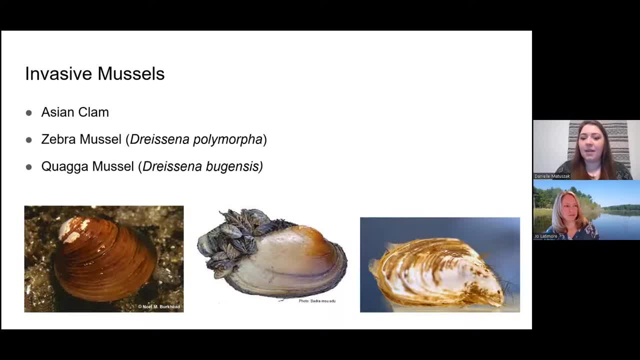 to describe it, facing down. That way it can open up from the substrate to filter feed. If you're not confident about your abilities to nestle it back in the substrate, simply setting it back where you found it In that same stream section as close to where you got it from. it's kind of that best practice That way you 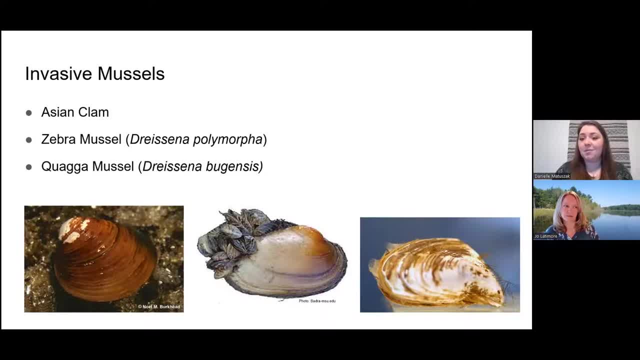 aren't moving it to an area that may not be suitable. So if you get one in one stream section and you put it 10 feet down the stream, that 10 feet can make a difference as to what that substrate is like. So again, 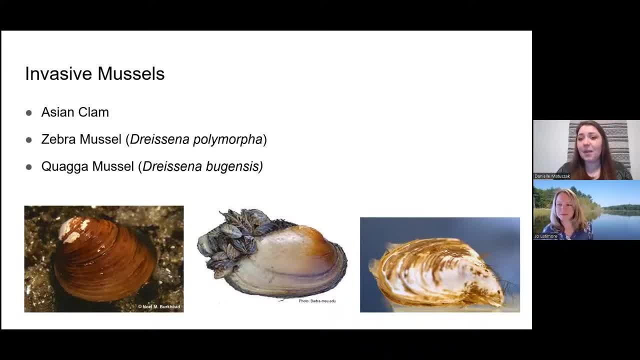 right where you find it. if you can remember where you found it, that's where you want to put it. Great answer, Danielle, And I'll add on To that from a MICOR perspective, our typical invertebrate sampling protocol suggests that you. 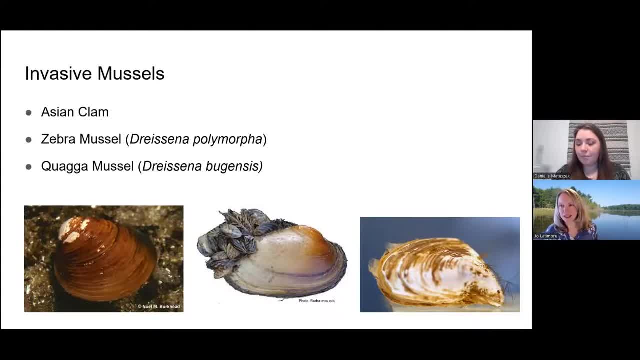 keep the invertebrates that you collect for later identification And as vouchers. we preserve them in alcohol and so forth. We make an exception for native mussels. If you encounter native mussels, following Danielle's advice for replacing them back where you found them is what we advise. 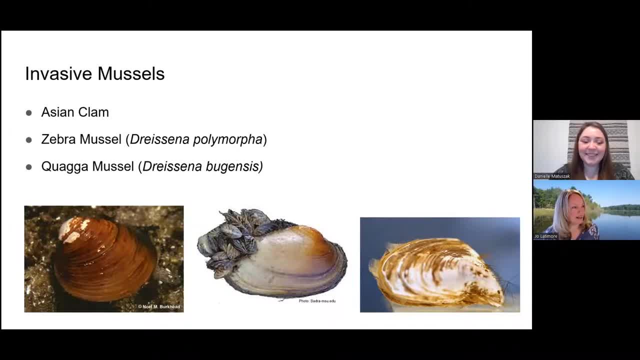 All right, Got a lot of questions coming in here. Let's see. Is there a limit to the size of the stream for mussels? I'm interested if mussels can be found in small headwater streams, maybe two to three feet wide, less than one to two feet deep. 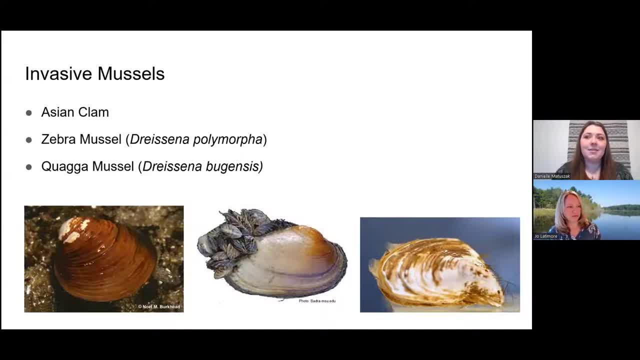 Good question. I am not entirely sure, So I there may be a specific species that is able to survive in that habitat. However, off the top of my head, I don't have a specific answer for that. There's a chance If there's other suitable habitat. if that stream is year round, it's a permanent waterbody. 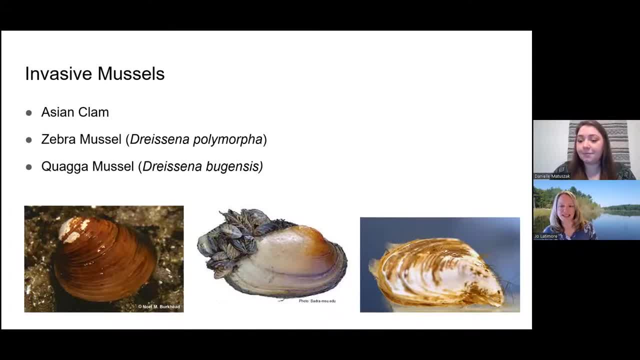 there's a chance that there might be All right. Thanks, Danielle, I'll remind people. if you have questions, please put them in the Q&A and not in the chat. We're looking in the Q&A for questions. Here's another question related to zebra mussels. What's the evidence for earlier? 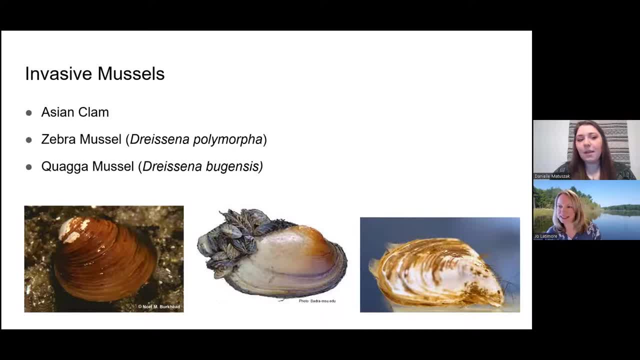 zebra mussel occurrence in North America. Do you have any insight on that? So yeah, it's super interesting And so I've done a little bit of research- not my specific research. I've done a little bit of reading into some of the literature that suggests that there may have been 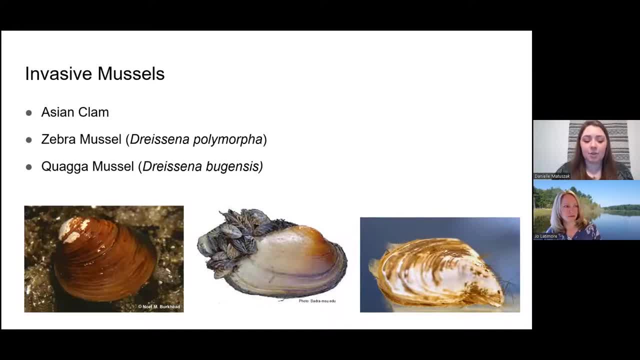 an earlier introduction And so basically they were able to do. I believe it's like genetic sequencing of I don't know what the exact- I'm not a geneticist so I don't know the names for all of these things- but there is some evidence that there's a potential. there's a potential. 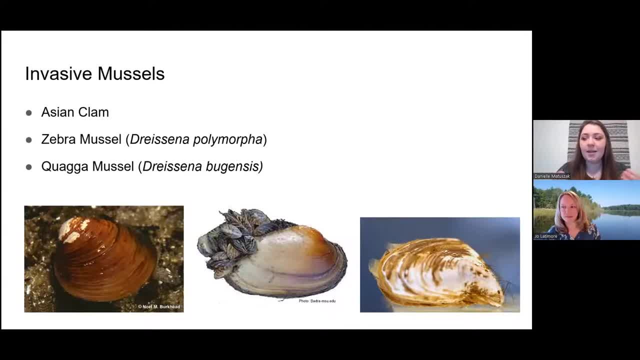 they were introduced earlier using some sort of sequencing from water samples and from zebra mussel like shells that they found that were deceased, that sort of thing. I don't know the specifics of how they did it, but I know that's in part a little bit of what they did Interesting. 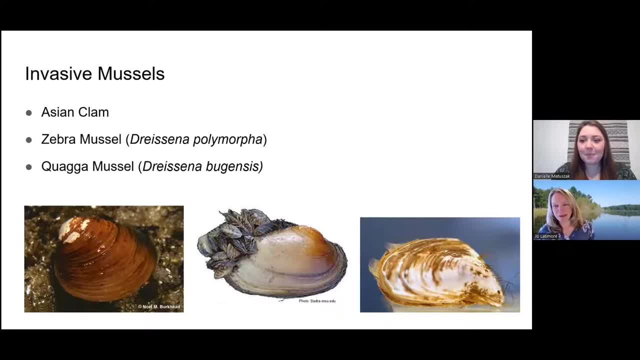 All right, One thing. there's a question that came in and it's about a topic that I know is really fascinating. is that reproductive cycle with the host fish and the and the, the glochidia that are released and attached to those gills? And one of our listeners wants to. 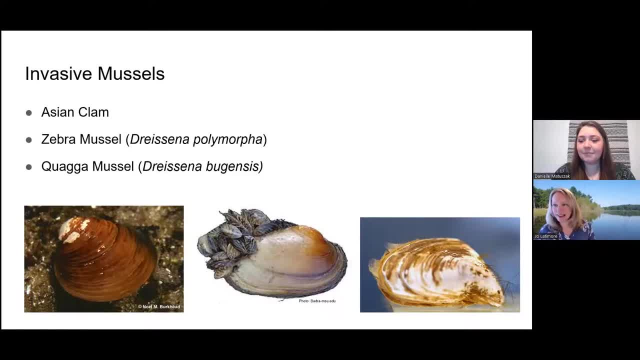 know? do those glochidia irritate the fish? Is there any kind of negative impact on their host fish? From my reading and understanding, typically not. There is actually some evidence that this parasitic phase actually protects that fish from other parasites that may want to attach to the 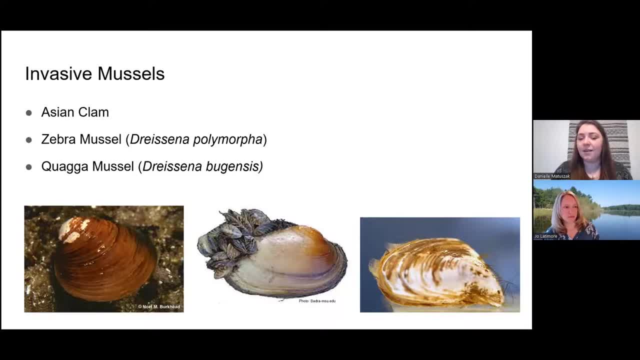 gills, simply because there's no more room if those glochidia are on there And it can help kind of strengthen that host fish or host fish species resistance to other parasites. I have not read any negative effects, Rather it's a symbiotic relationship. So that is where you know both. 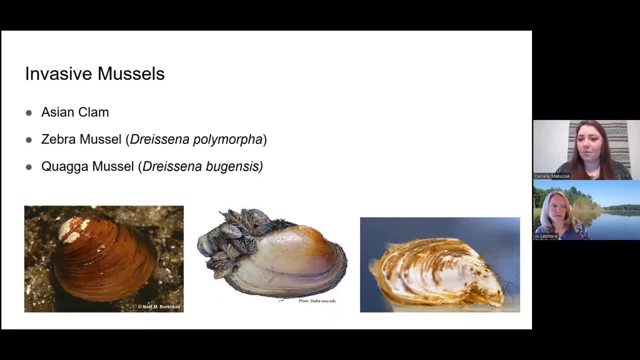 parties, or at least one party benefits from that relationship. All right, Thank you. Lots of questions coming in about zebra mussels. I don't know if we'll get to all of them, but I'll. I'll ask a couple. 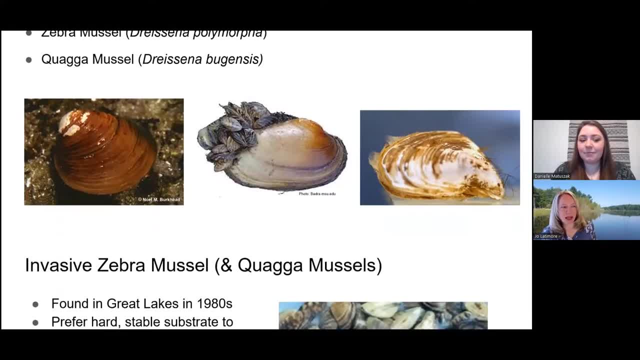 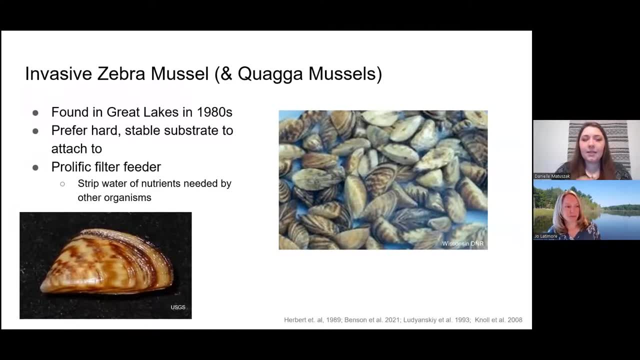 This listener says: I might've missed you saying this, but has it been discovered why zebra mussels survive by attaching to other mussels? So it's not that they specifically will attach to other mussels. It's the second bullet point here on the slide that I just brought up, that they prefer hard, stable substrate and some. 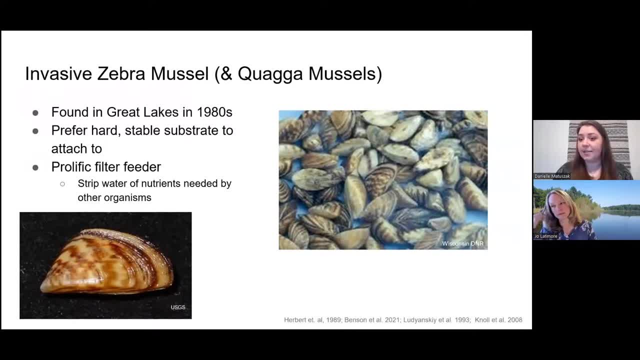 freshwater mussels. once they're adults, they don't move. They stay in the same area. It's not for all species, but some species do. So the shells of those freshwater mussels are hard, And if they're the kind of species that doesn't move around, they're quite stable, And so it's. 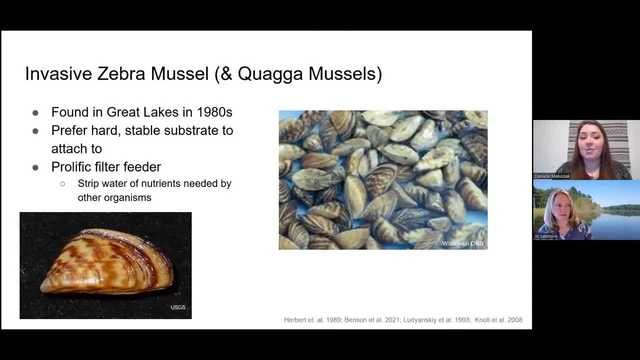 simply that they're not necessarily targeting freshwater mussels. It's just that they happen to make up the kind of substrate that they like to attach to. All right, We're going to go more broadly now into lakes. A person asks: we have sedimentation. 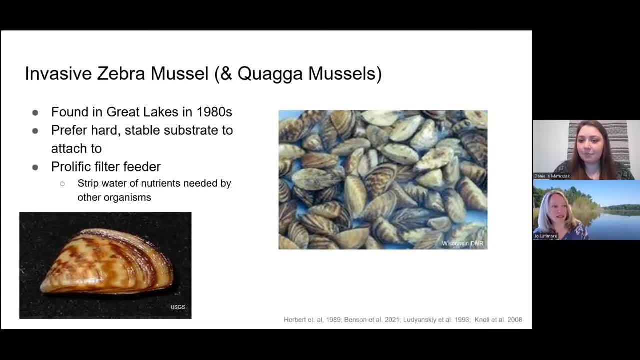 in our canals and on our lake. So there's sedimentation in the canals on their lake and they're considering dredging those canals. Sounds like both can be a problem for mussels- both the sedimentation and the dredging. 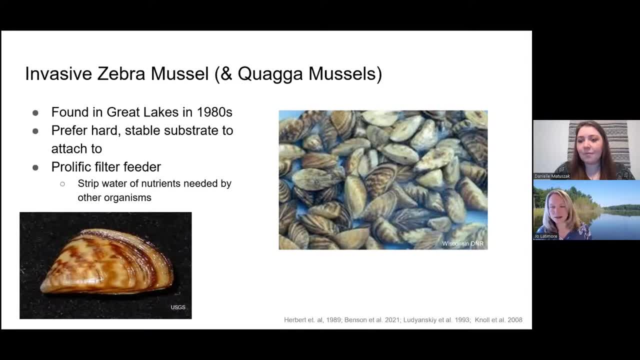 Are there guidelines for dredging that can have the least effect on mussels? So I'm not super informed on the specifics of guidelines, but in many cases when there's dredging occurring, removal of dams, there's a lot of regulations that are have been developed or 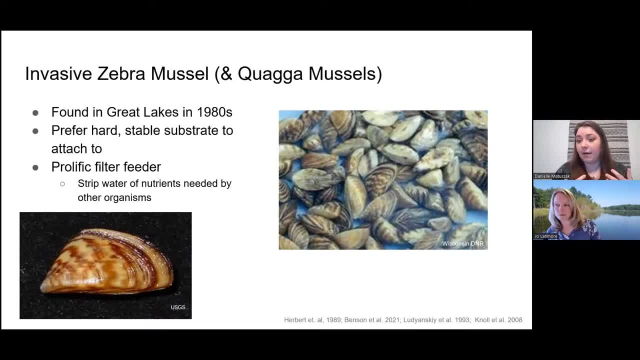 are being developed to make sure that they're removing any mussels that they find doing the dredging, doing that sort of thing for remediation, or whether they need to deepen the channel for navigation or something, and either putting those mussels back or moving those mussels to a similar ecosystem that that species has been known. 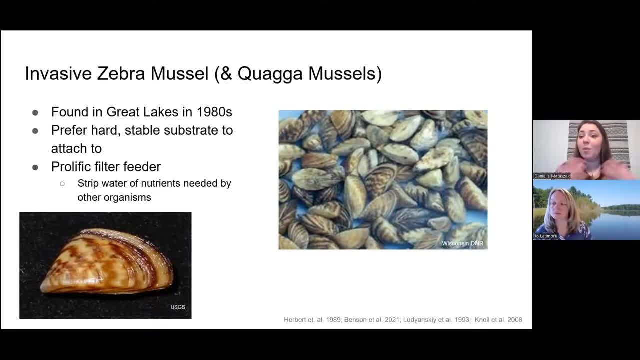 to survive in. There is a lot more specifics and nuances to that, a lot more politics and policies that go into that, many of which, I believe, can be found on the Michigan DNR website. There's some regulations that are listed publicly there. 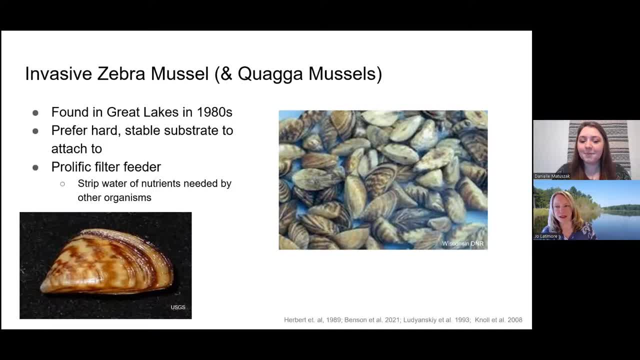 Right, Absolutely, Absolutely. Great answer, Danielle, And I think another thing that I would mention along those lines is that if you're planning a project, a dredging project or other projects that may require disturbance of the bed- the lake bottom stream bed, that kind of thing, you know- it can be a good idea to do a survey of mussels there to see if you may be in an area that would be disturbing the habitat of mussels that are there. 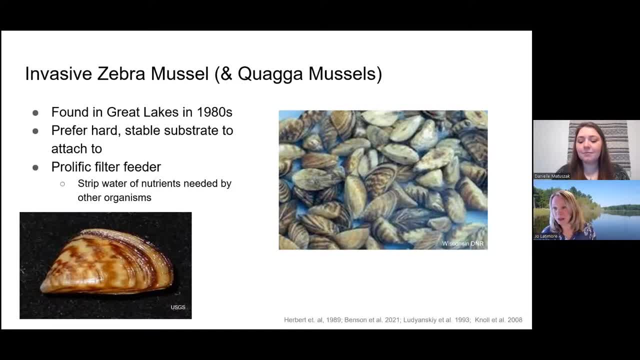 Because they tend to be one of those groups that don't get a lot of attention or notice, because you don't really see them very easily unless you're looking for them. So I'm glad folks are thinking about it. Staying in lakes: Danielle, do you have any more details or information about endangered mussel species that live in Michigan's lakes? 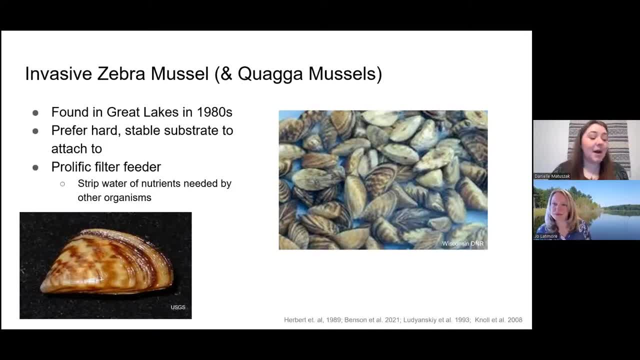 I do A little bit. So the pocket guide that I mentioned, so I have a copy, a hard copy- of it here And it lists many of the kind of endangered species that are in freshwater for freshwater mussels. However, a lot I believe the Michigan DNR as well as like the USGS with their endangered species database, can kind of identify the endangered species there. 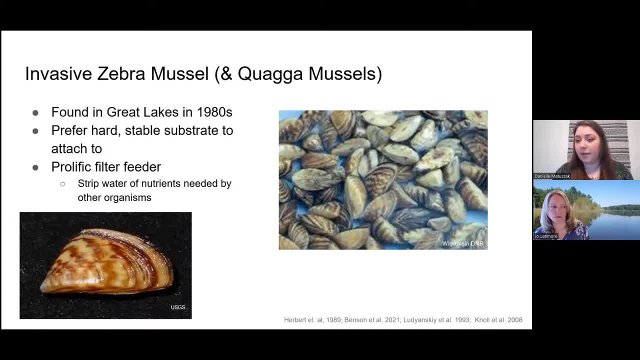 And both of those websites, I believe, have ways to identify those mussels in your lakes or streams as well. All right, Thank you. Thank you, All right. Questions keep coming in. We've had a couple that connect zebra mussels and algae blooms. 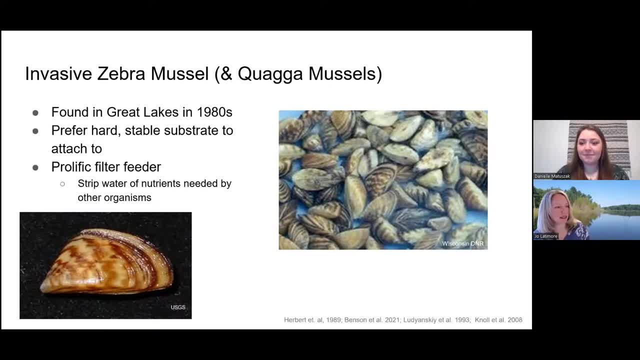 For example, here's one that specifically says: can you discuss in more detail the impact that zebra mussels has had on aquatic environments, especially as they relate to algal blooms? Yeah, so I definitely can. I won't get too in depth, so we always have time for more questions. 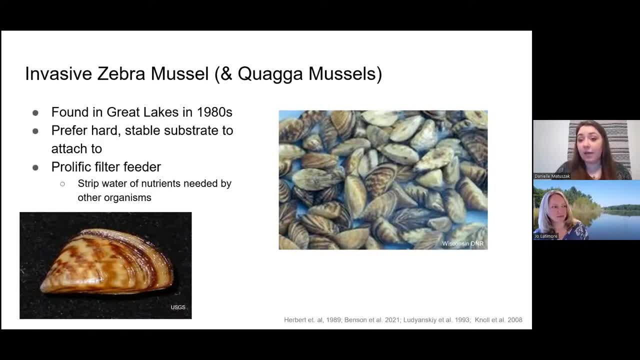 But basically there has been links to harmful algal blooms And this prolific filter feeding of zebra mussels and, in turn, quagga mussels. So I don't know if any of you have heard of microcystin, that toxin that has also been tied to these algal blooms from that blue-green algae. 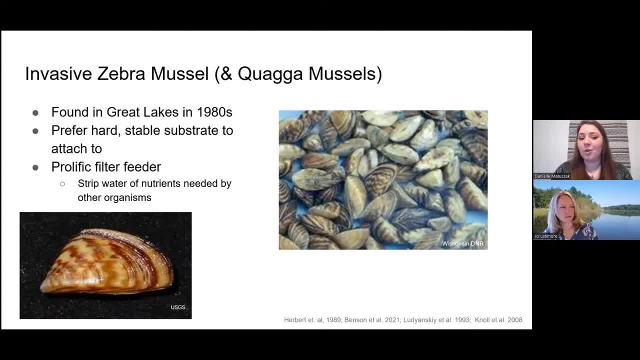 Basically zebra mussels. they're, also, besides being prolific, are also preferential. They're picky eaters, And so what they will do is they will intake their water to filter feed, take out all the goodies that they want and then spit back out. 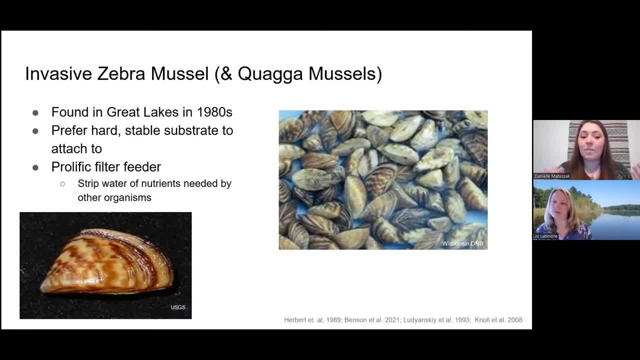 What they don't want, And a lot of times that is microcystin. And so with these harmful algal blooms you can kind of get this abundance of microcystin building up in the water, which is just a very brief general way to describe kind of what happens. 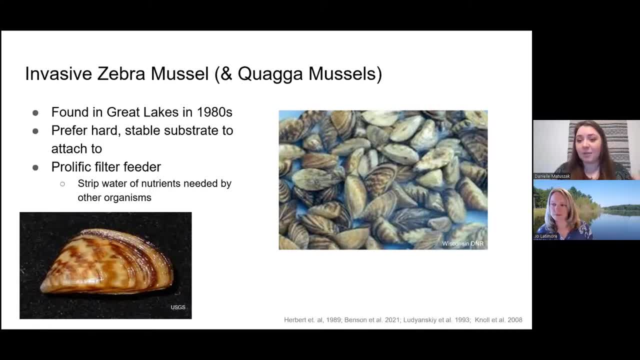 But yes, you can have these harmful algal blooms that can cause sickness in fish, pets, humans. That's why a lot of times during the summers you'll see, you know, signs along lakes that if it's green, Don't go in because of those harmful algal blooms. 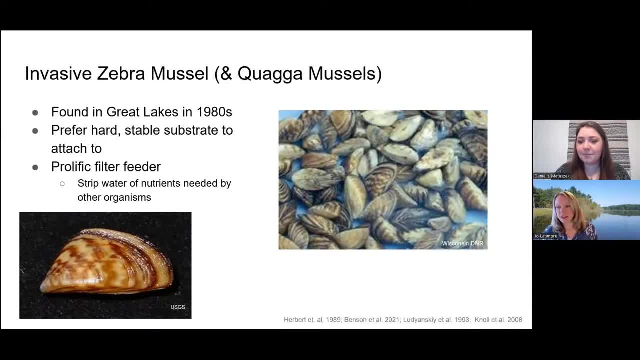 Hopefully that answered that question a little bit. Absolutely, It actually answered a few people's questions. That one came up a lot On the flip side, though, related. Do you know, has it ever been documented that a bad algae bloom could actually hurt the mussels like hinder, native mussels that are living in a water body? 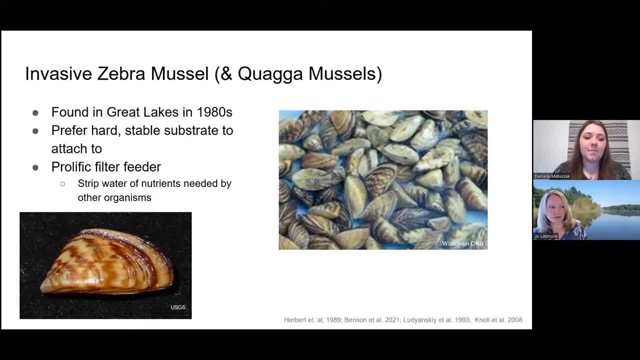 I personally don't know the specifics of that. I do know that If there is that accumulation of microcystin, that potentially could hurt the native species and actually can form what's called bioaccumulation. So if it is absorbed into the body tissue of mussels of fish, as other fish predate upon those mussels and fish, and it goes up through the food web to the fish that us humans eat, we can get sick sometimes from eating that. 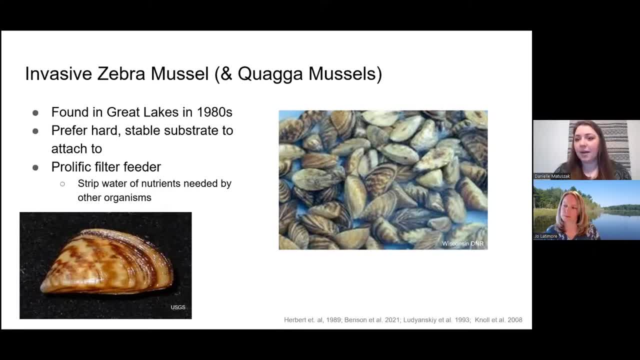 So it's not directly answering the question, but it can in turn, I believe, Have some impact on native species, though I don't know the specifics of it. Understood, Yeah, great, And I'll mention to folks that we do have several folks from DNR and EGLE in the audience today and they've been helpfully adding some information about dredging projects and permits and all that stuff and also addressing some of the other questions in the chat. 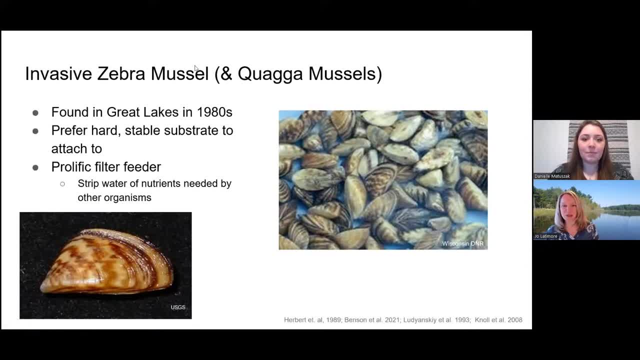 So take advantage of that and take a look at the chat, folks, if there's a bit more information there. And obviously the topic of mussels is very, very broad, And so we'll do the best we can between between our guest speaker and our audience members to get your answers while we're here today. 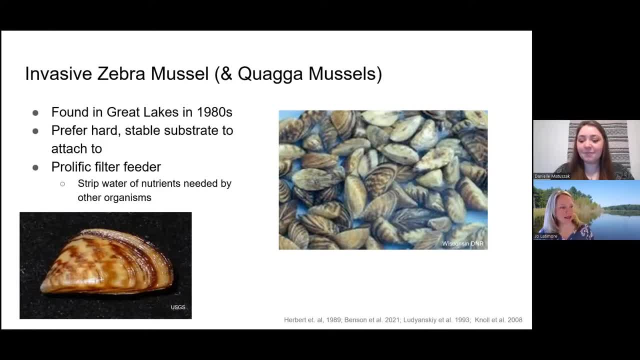 We've got about ten more minutes, And so I'm going to look at a couple other questions that have come in. If you were to speak to a waterfront homeowner, a lakefront homeowner, a streamfront homeowner, you know what would you say to them as an individual? 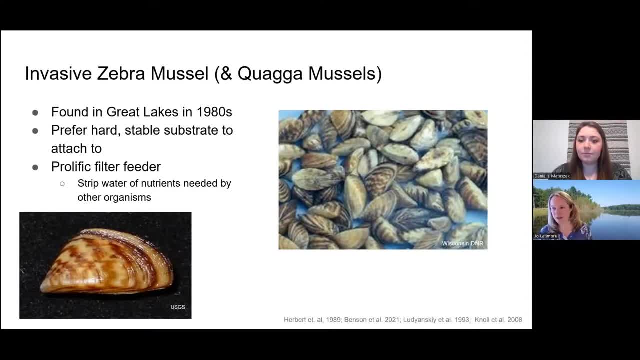 What could they do personally To help protect the native mussels that may be found in habitat near their their own property? Yeah, that's excellent. So I actually have family members that are lakefront owners and we found mussels off the side of their docks. 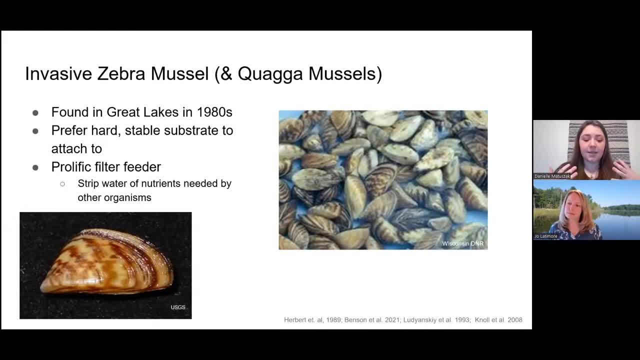 And one thing that I told my- even my- family members is that if you find the mussels, don't move them. Do your best to avoid disturbing them. If you have, if it's in your lake, but not necessarily On your property or on your section of lake, talk to the other people, your neighbors. 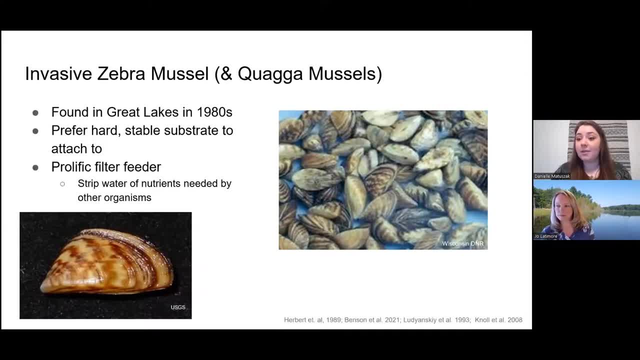 If there's other people that are living on your lake or stream, about making sure that they're not moving them. If you're doing stream walks, where you're walking through the streams to avoid those areas, And the best kind of arsenal I can recommend is making people aware that they are there and also making them aware of the fact that it's illegal to take them to leave. 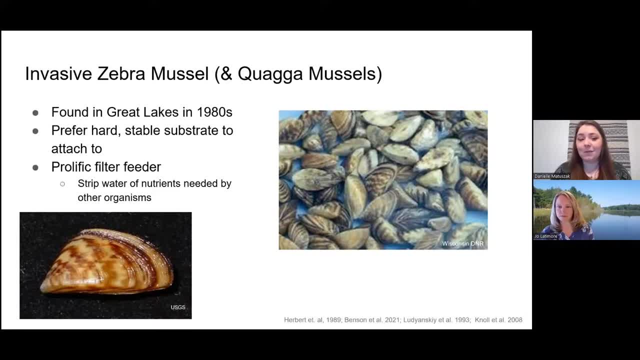 You want to leave them there so that they are able to help maintain that ecosystem. So those are kind of the in general recommendations I would give All right thanks, Here's a great one. I love this one. What's your favorite mussel and why? 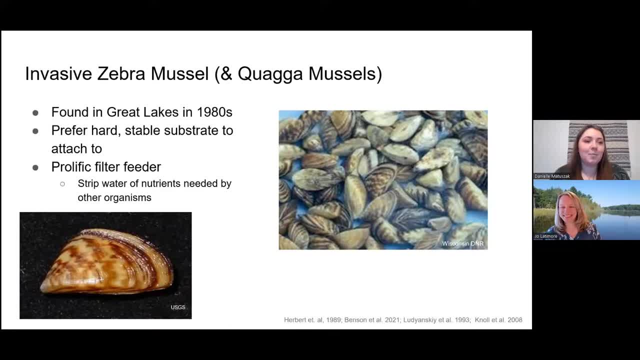 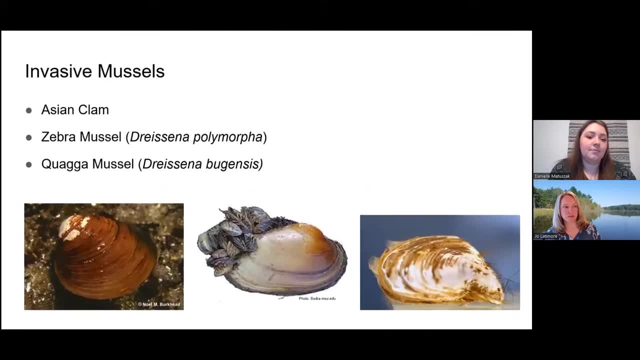 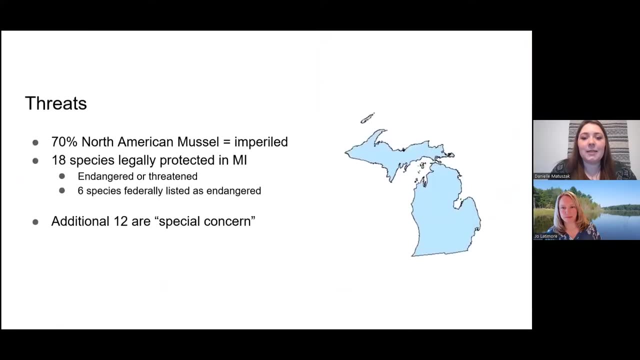 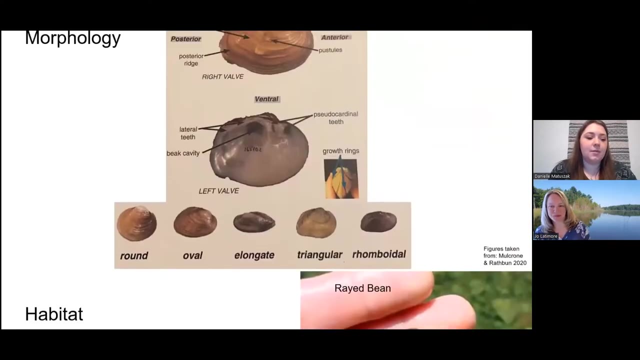 That's. that's tricky Personally. I think I have it on a previous slide here. I think I have that Go all the way back, So it's a little bean of a muscle. I think it's absolutely adorable. There was. 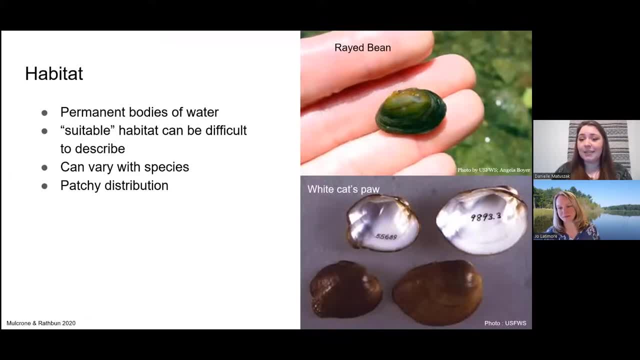 This raid bean. I think they're absolutely adorable. They're so little. They're like this big, As you can see by the size scale for the image there. I think they're really cute. the little mussels: I think they're adorable. 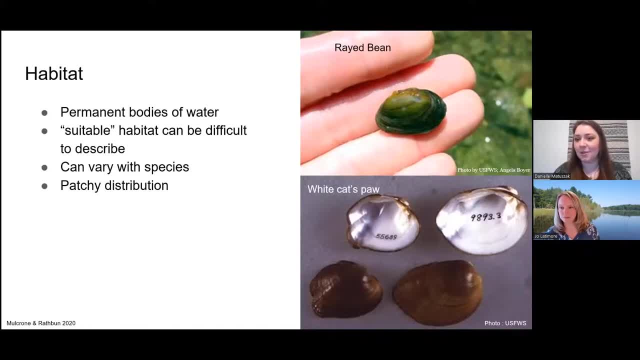 but also white cats. There's a reason these two were in the slides. I think they look- I don't know. they look kind of funny with their little knob on one side. I would say those are my favorite. but I'm also not, you know, exposed. I have never been exposed. 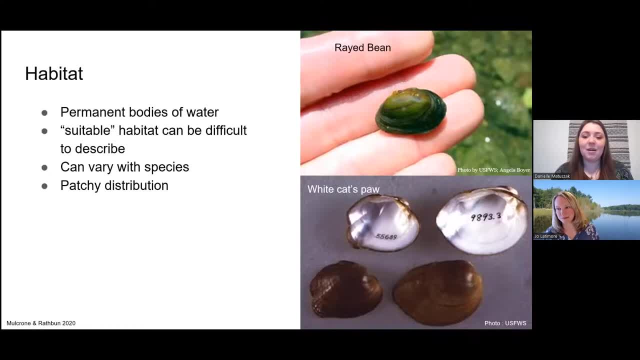 to all of the freshwater mussels in Michigan. so of the ones that I've seen, or of the ones that I've researched or looked into a little bit, these are two. These are also like I mentioned. they're imperiled or endangered, but I don't know. I like all mussels. They're kind of cute. 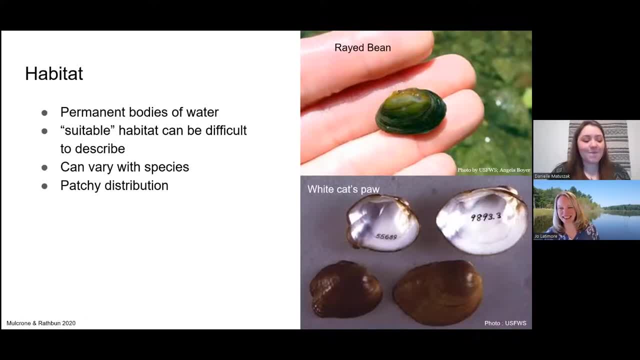 Yeah, they really are, and I love the names. right, There's some really great common names for our freshwater mussels. Yep, there's a wide variety of names, Everything from- you know- the rayed bean to the pimpleback, to the doe foot- I believe is one of them. 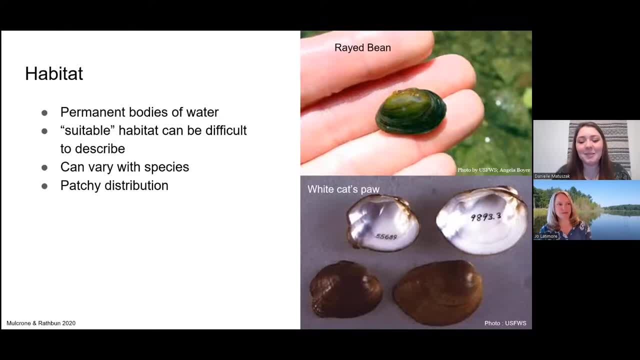 Yeah, fluted shell, the names are quite fun. We've had a couple questions come in about how long native mussels live. Do you have any information on that? There's some suggestion that some might be quite long-lived. Yeah, so it can vary by species, As with. 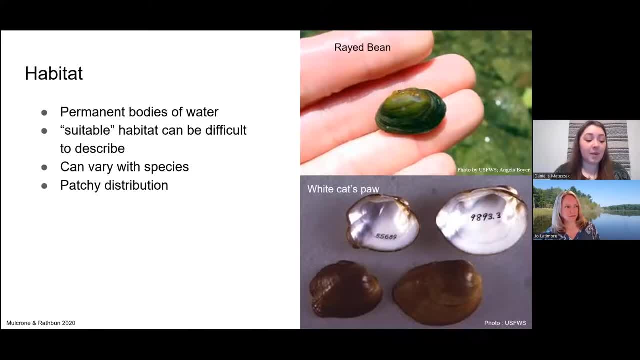 kind of the way that organisms go, but they can live decades long. so you know, if you find a very large mussel- I mean it's not always indicative If it's a smaller species- you aren't going to find a mussel the size of your fist if the species only gets to be two inches long. but 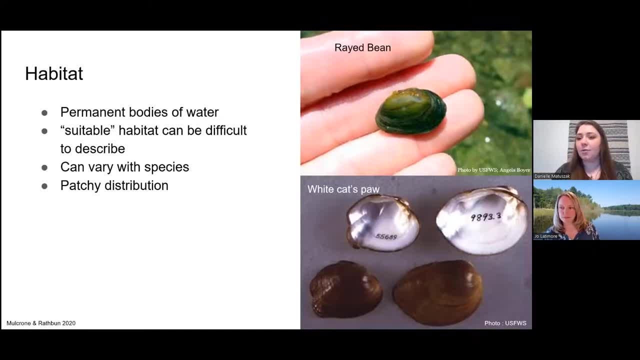 in some cases you can see kind of those rings and the growth rings in the image that I have back here. You see growth rings, It's kind of one or two. I'm just doing some Fermi motion and then it's kind of another thing I'm going to do. 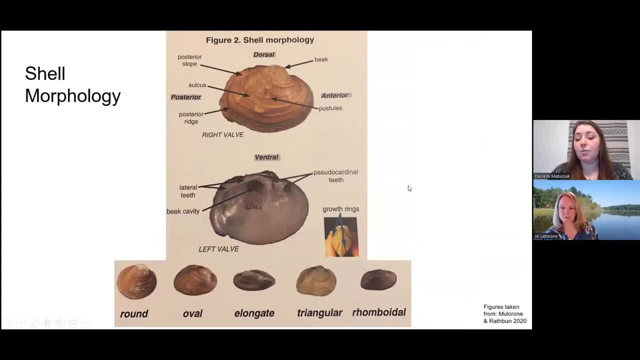 away with. You've got, like almost every species, Telod entrance of the heat flux area, but even the completion sideral development here on that bottom right of that morphology image, And so those growth rings can help you tell how old that muscle is. I don't know what the oldest muscle was recorded That would be. 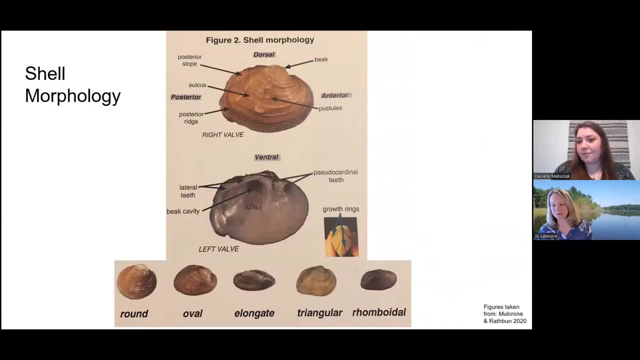 very interesting fun fact, but that's how you can kind of tell. but they can live to be quite old, decades at the very least. in some cases Absolutely. And in fact, the pocket guide book that you mentioned, one of the authors, Joel Rathbun. he's in the audience today and he just 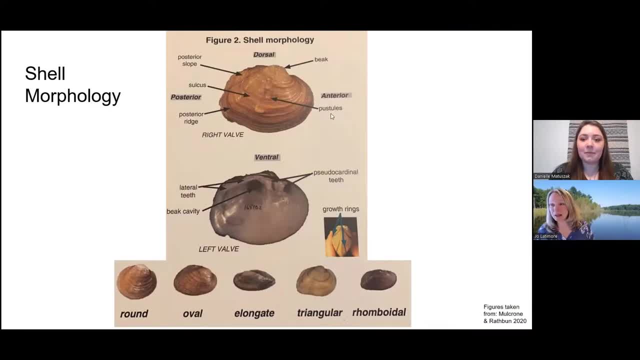 typed in the Q&A that they can be up to 180 years old. Isn't that amazing to think about that? some little clam that you run across in a river could have been in that water body for so long. It's pretty amazing, And it also kind of gets at the importance of keeping habitat and water quality. 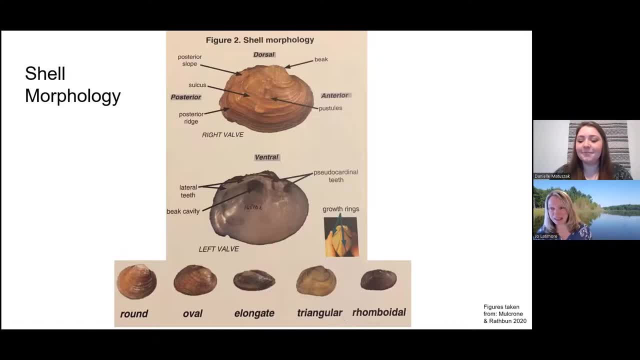 good, over a long period of time, for them to really meet their lifespan, which is really kind of mind-blowing, isn't it? Oh right, Right Back to the reproduction. You started to talk a little bit about this, but there's also 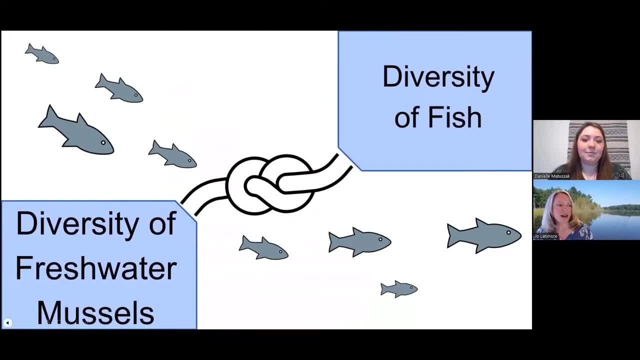 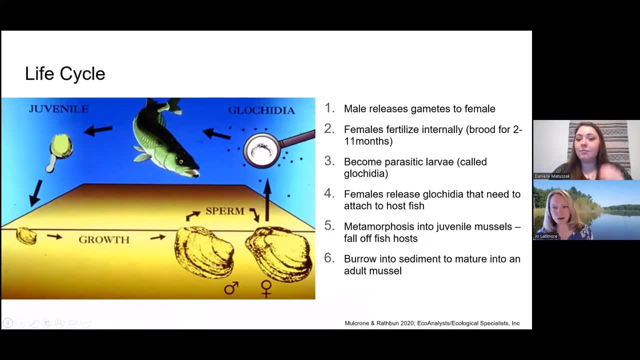 some folks that are really interested on more. Are there certain species of host fish that the mussels connect to? Is that a specific relationship between a particular mussel and a particular fish species, or how specific is that relationship? It depends on the species. I know that seems to be the answer for a lot of it, but 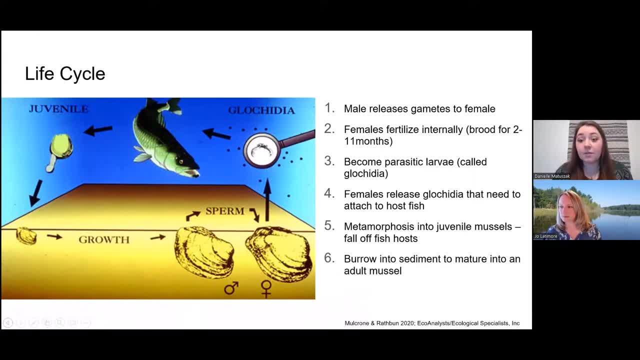 sometimes Some species have several fish that they can use as host fish. Some even use salamanders, But in general it's typically a fish. Some species can only use one, maybe two species of fish, So if that fish species is not there they're not able to reproduce. So it varies by species, but some can use several different host fish. Others are very specific to a singular species of fish. 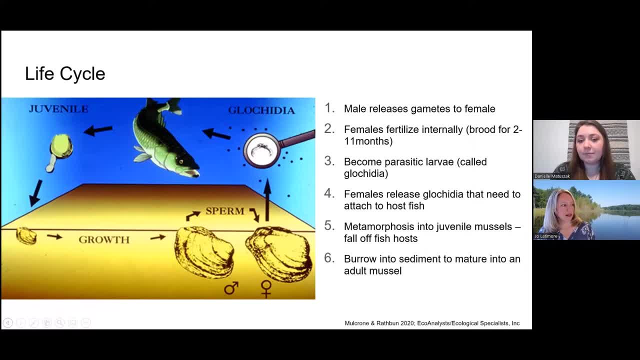 Great, Thank you. Thank you, We did have. we have had a couple people ask about getting a copy of the pocket guide And I know I've spoken with Joe about that recently And, Joe, if you have insight on that, feel free to to comment. But I would also say I know we do have an example of the PDF version of that And we could actually we're going to post the recording of this webinar and we could post a copy of the. 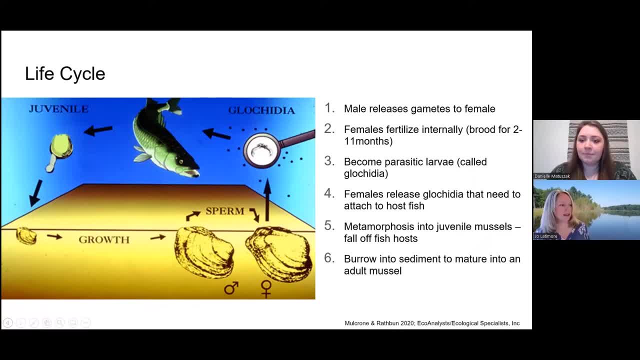 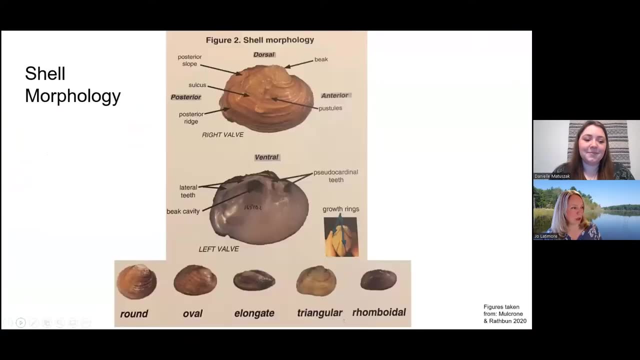 PDF There for people to access it. Let's see, we've got just a couple more minutes, So I'm going to look for. Oh gosh, I know we're not going to get to everyone's questions. So, Danielle, maybe if you want to scroll back to your contact information on that last slide, if people want to follow up with you, I'm looking for one. that another kind of popular theme here. 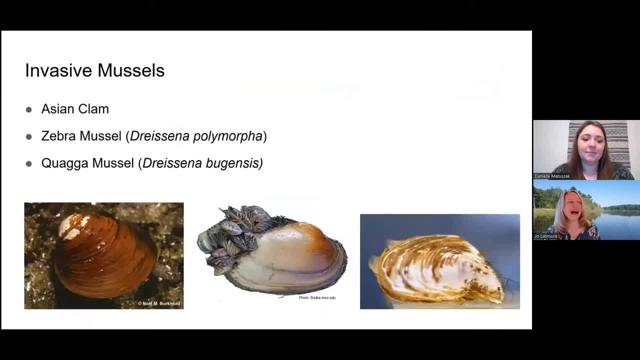 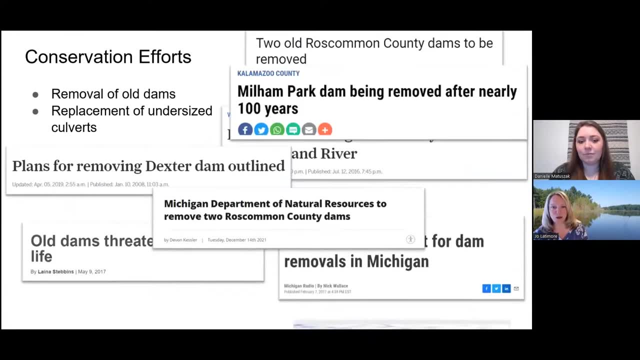 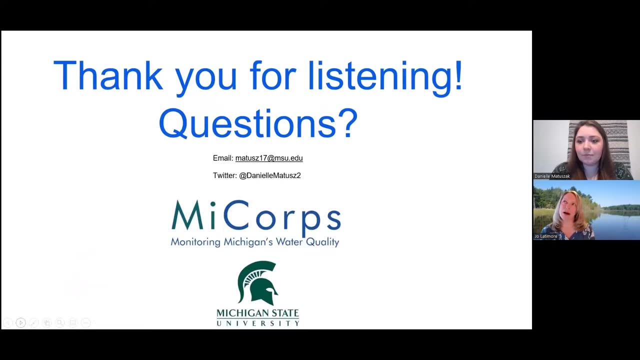 Let's see. Ah, we've had a couple of questions, A couple of questions related to native mussel restoration after you know habitat damage has happened or after zebra mussels have come in. Could you say anything about like reintroduction of native mussels into an area especially you know? can can mussels be farm raised or raised in a hatchery and and reintroduced and if, if, if that is possible, or transplanted? 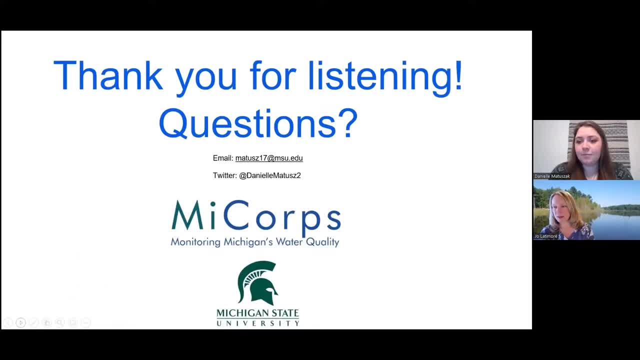 Can glyphosate be? Haha? And if you're, lake has zebra mussels in it, should you bother? So for the second half of that question of zebra mussels and should you bother, it's going to depend on the lake, it's going to depend on the ecosystem. but for the first half of that question about you know kind of lab growth of muscles and kind of reintroducing into up, 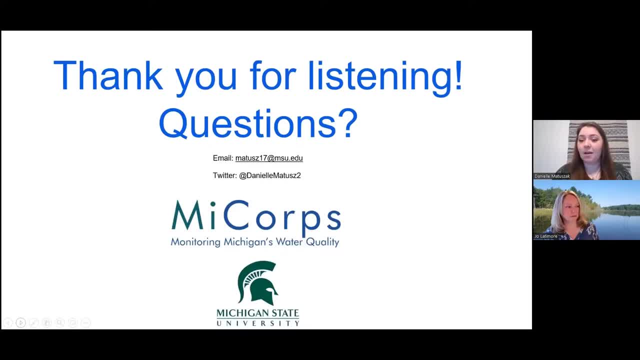 Yeah, the last time I heard you I was watching with a good friend that said: I just want to go to this and into. I know I believe it also has been done in North Carolina or they were planning on doing it in parts of North Carolina, So it has been done. I do not know the results of how well those 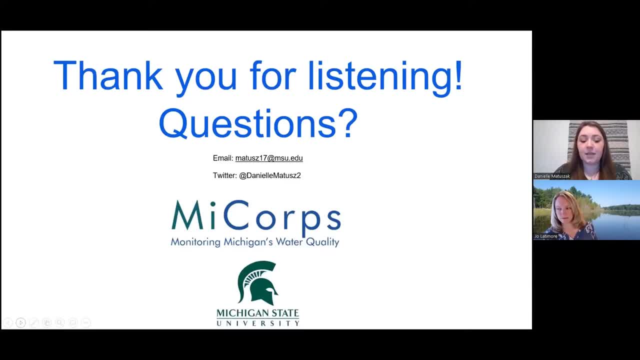 populations maintained. but it's been done So they are able, some species are able to have they be raised in a lab setting or in a hatchery setting. Again, a key thing with that is having that host fish. So it's not just raising that muscle, You also have to raise the host fish. that 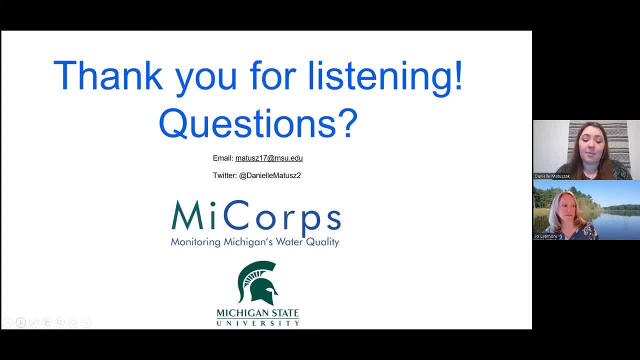 goes along with it, which can make it quite intensive, because you need to have habitat that's suitable for both within your hatchery or your lab. It has been done. I do not know the extent of how well it is done, as well as how sustainable that process is. So the inputs of 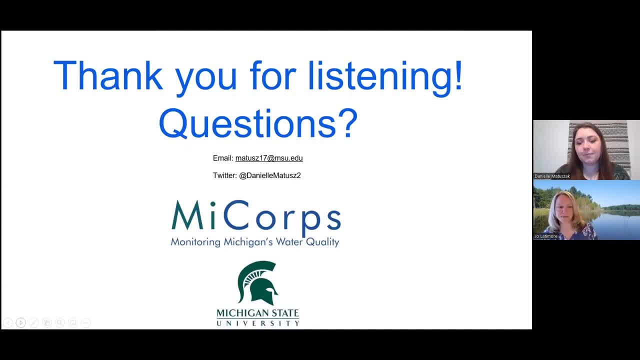 the cost effectiveness. effectiveness, all of those things. All right, Danielle. thank you so much. I wanted to wrap up with a couple of comments I did just put in the chat. One of the co-authors of the pocket guide, Joe Rathbun, provided his email address, So if you're interested in getting a copy of that, 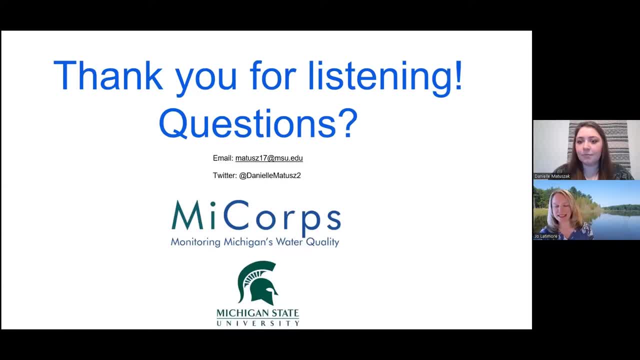 refer to the chat, rathbunjsbcglobalnet. You can contact him and he will do his best to get you connected with a copy of that pocket guide. I know I have a couple of copies myself and it is a really, really fun, interesting reference specific to Michigan, which is great. 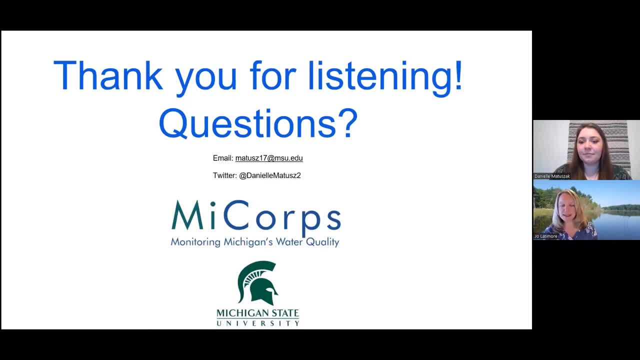 I also wanted to remind folks that this was recorded. This will be once we clean up the recording and it gives us a little time- maybe give us a week or so- we will post it on the same page. you went to to register at mycorenet, Visit there and under the description of Danielle's, 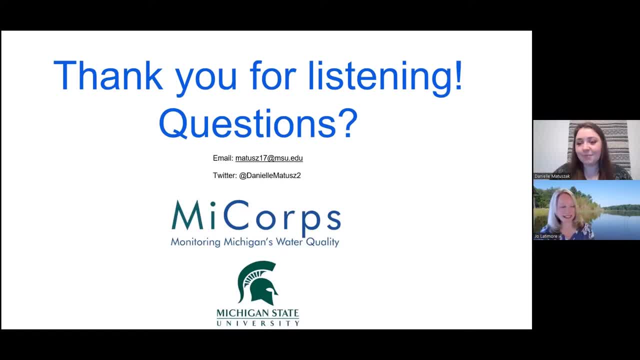 presentation. a link to the recording will appear in about one week. I also wanted to remind folks that this is just the first of a series of webinars that were organized by Danielle primarily, So we thank her for that as well. Our next one will be on the next.